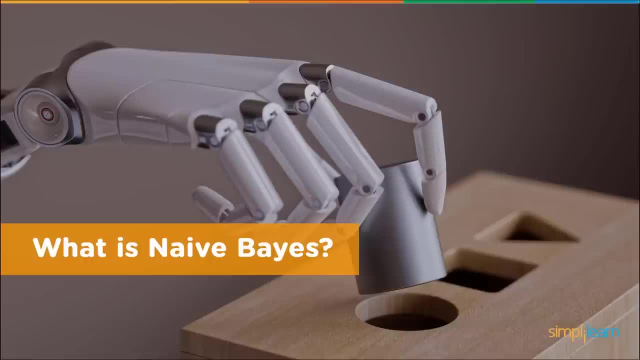 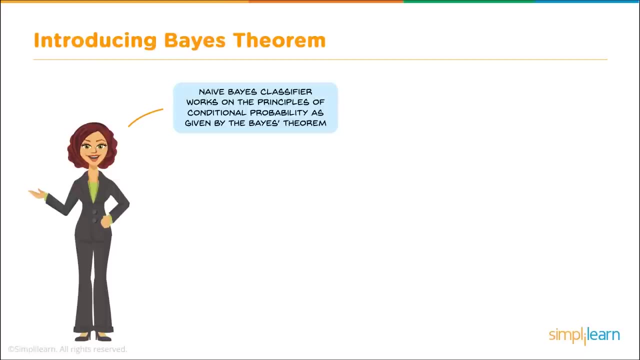 classification using the Naive Bayes. What is Naive Bayes? Let's start with a basic introduction to the Bayes Theorem, named after Thomas Bayes from the 1700s, who first coined this in the Western literature. Naive Bayes Classifier works. 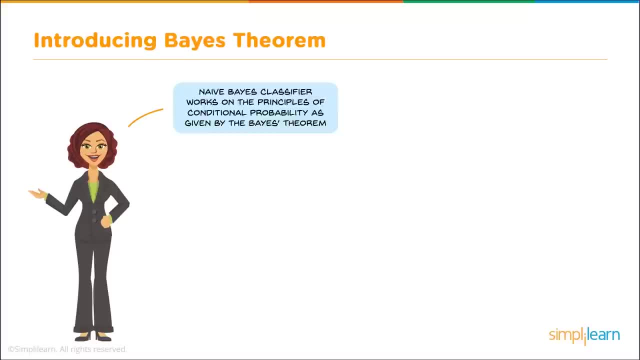 on the principle of conditional probability as given by the Bayes Theorem. Before we move ahead, let us go through some of the simple concepts and the probability that we will be using. Let us consider the following example of tossing two coins. Here we have two quarters and 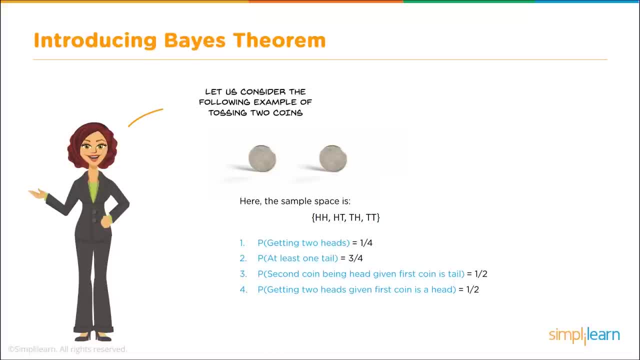 if we look at all the different possibilities of what they can come up as we get that. they could come up as head, heads come up as head, tell, tell, head and tell, tell. When doing the math on probability, we usually denote probability. 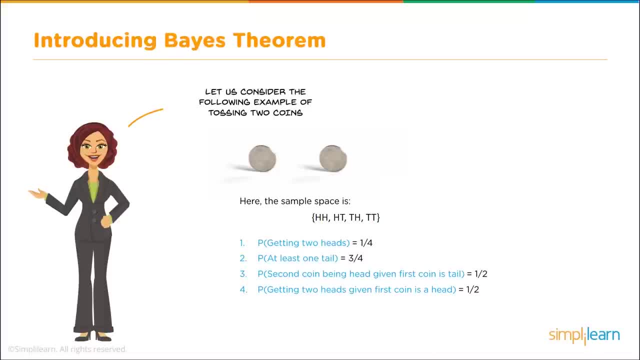 as a P, a capital P. So the probability of getting two heads equals 1: 4th. You can see on our data set we have two heads and this occurs once out of the four possibilities. And then the probability of at least one tell occurs three. 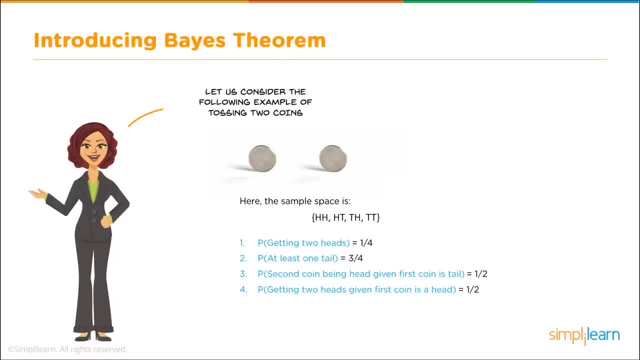 quarters of the time. You'll see on three of the coin tosses we have tells in them And out of four that's three fourths And then the probability of the second coin being head, given the first coin is tell is one half and the 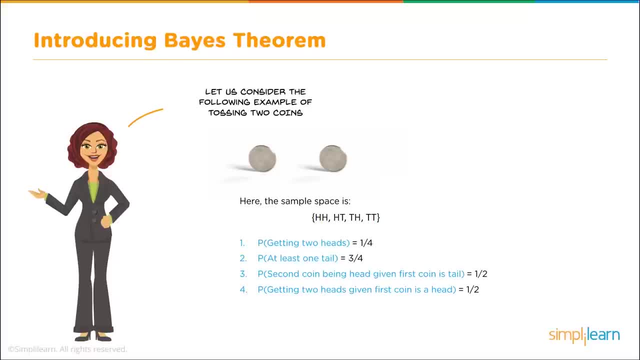 probability of getting two heads. given the first coin is a head is one half. We'll demonstrate that in just a minute and show you how that math works. Now, when we're doing it with two coins, it's easy to see, but when you have something more, 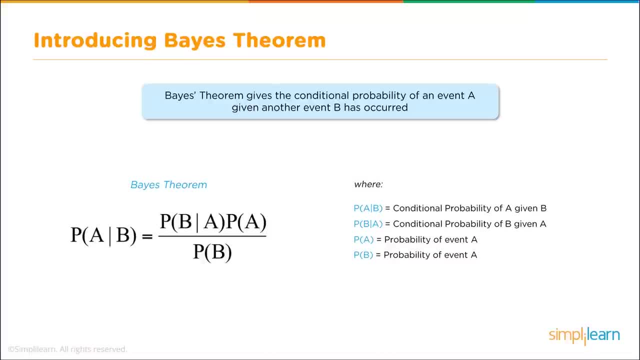 complex, you can see where these formulas really come in and work. So the Bayes Theorem gives us the conditional probability of an event A given another event B has occurred. In this case, the first coin toss will be B and the second coin toss A. This could be confusing. 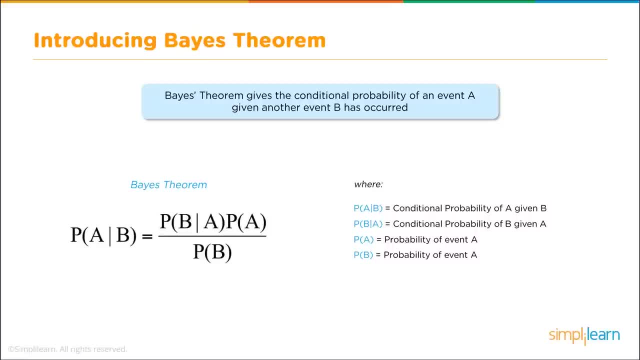 because we've actually reversed the order of them and go from B to A instead of A to B. You'll see this a lot when you work in probabilities. The reason is we're looking for event A. We want to know what that is, so we're going to. 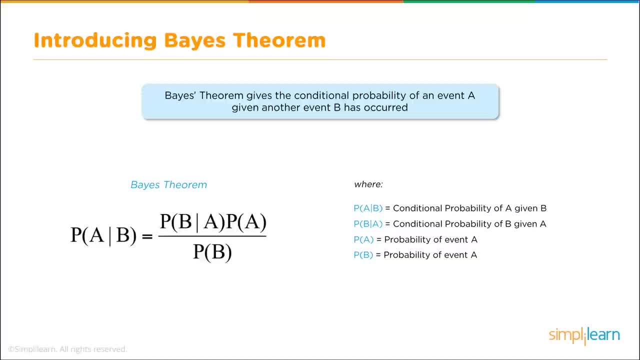 label that A, since that's our focus. And then, given another event, B has occurred. In the Bayes theorem, as you can see on the left, the probability of A occurring given B has occurred equals the probability of B occurring, given A has occurred, times the probability of A over the probability of B. This simple formula. 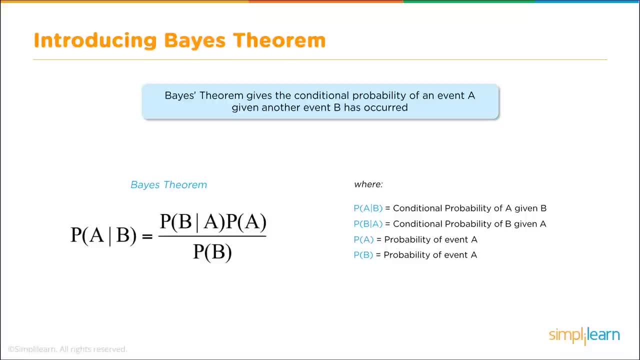 can be moved around just like any algebra formula And we could do: the probability of A after a given B times probability of B equals the probability of B given A times probability of A. You can easily move that around and multiply it and divide it out. Let us apply Bayes theorem. 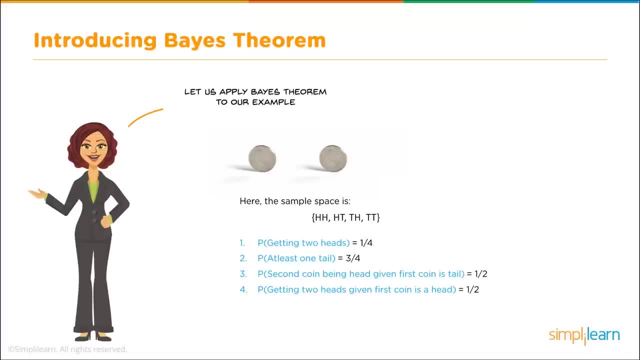 to our example. Here we have our two quarters And we'll notice that the first two probabilities of getting two heads and at least one tail we compute directly off the data. So you can easily see that we have one example, HH, out of 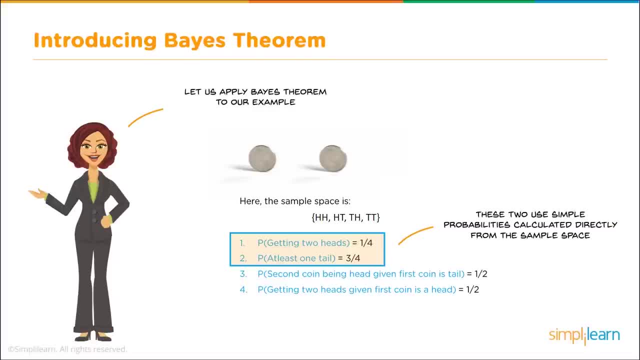 four, one fourth, and we have three with tails in them, giving us three quarters or three fourths- 75%. The second condition, the second set, three and four. we're gonna explore a little bit more in detail Now. we stick to a simple example. 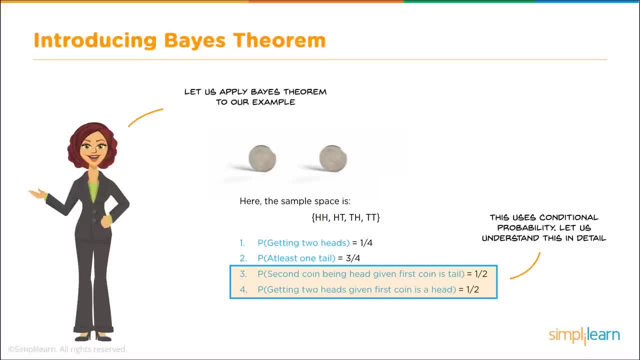 with two coins, because you can easily understand the math. The probability of throwing a tail doesn't matter what comes before it and the same with the head. So it's still going to be 50% or one half. But when that probability gets more complicated, let's say you have a- 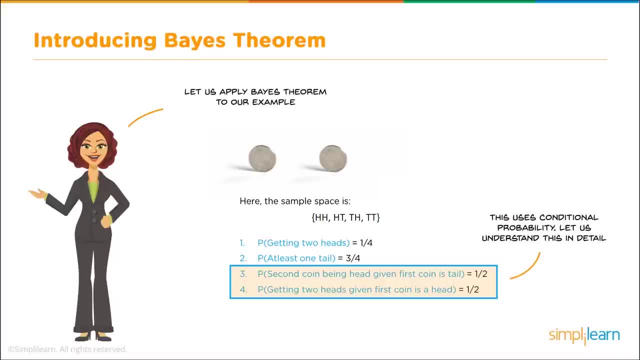 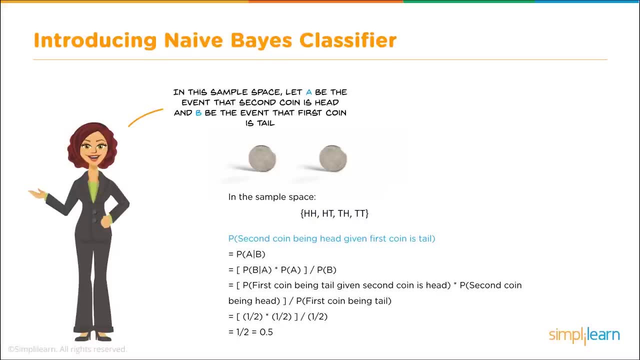 d6 dice or some other instance, then this formula really comes in handy. But let's stick to the simple example for now. In this sample space, let A be the event that the second coin is head and B be the event that the first coin is. 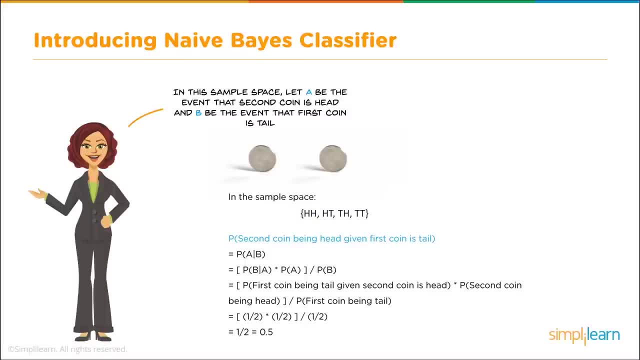 tails Again. we reversed it because we want to know what the second event is going to be. So we're going to be focusing on A And we write that out as the probability of A given B, And we know this from our formula that that. 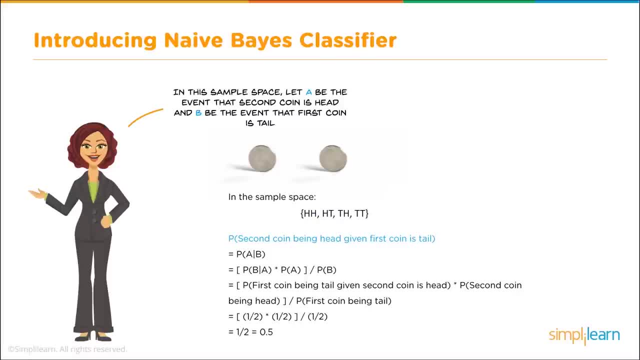 equals the probability of B, given A times the probability of A over the probability of B, And when we plug that in, we plug in the probability of the first coin being tails, given the second coin is heads, and the probability of the second coin being heads, given the first coin being over the probability of the. 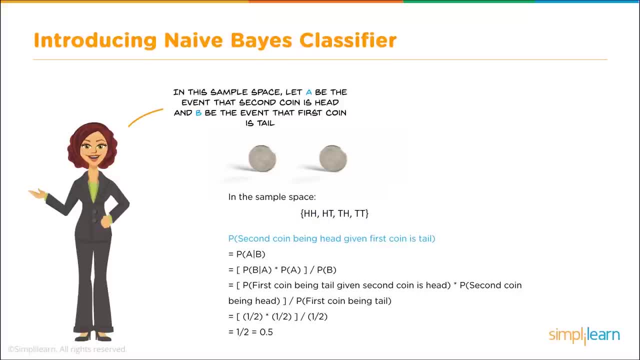 first coin being tails. When we plug that data in and we have the probability of the first coin being tails, given the second coin is heads times the probability of the second coin being heads over the probability of the first coin being tails, You can see it's a simple formula to calculate. We have 1. 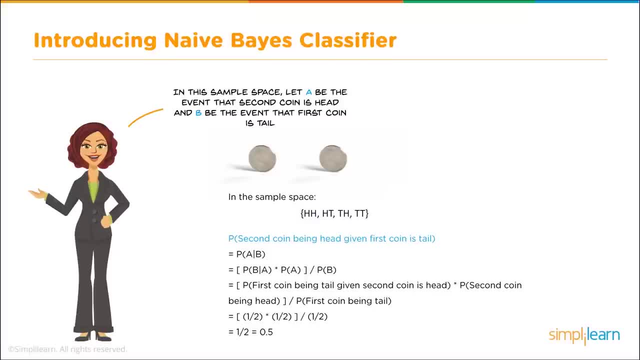 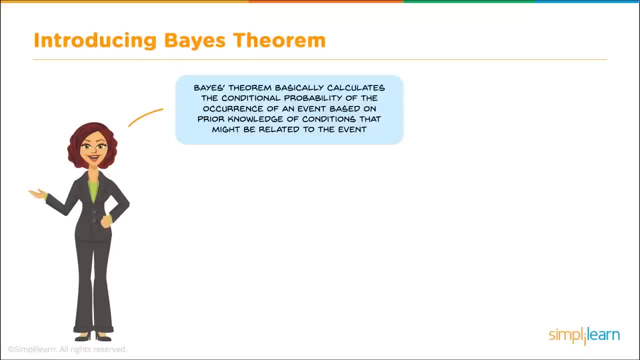 half times 1 half over 1 half, or 1 half equals 0.5 or 1 fourth. So the Bayes theorem basically calculates the conditional probability of the occurrence of an event based on prior knowledge of conditions that might be related to the event. We will explore this in detail when we take up an 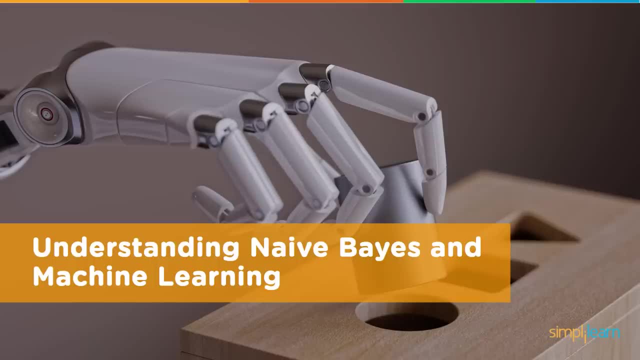 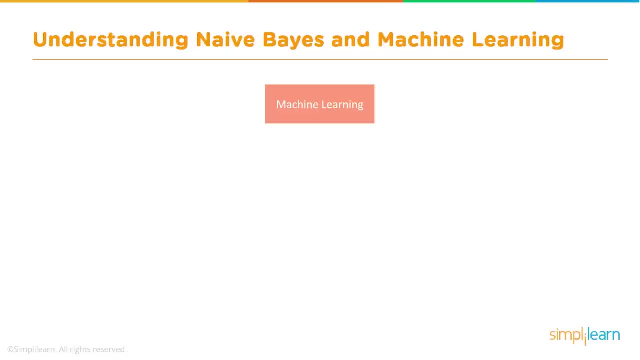 example of online shopping. further in this tutorial, Understanding naive Bayes learning. Like with any of our other machine learning tools, it's important to understand where the naive Bayes fits in the hierarchy. So under the machine learning, we have supervised learning and there is other things like. 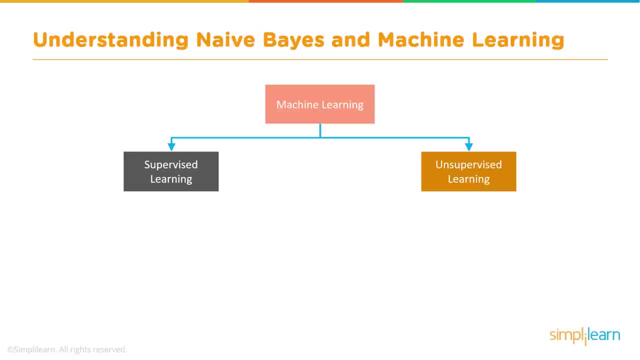 unsupervised learning. There's also reward system. This falls under the supervised learning. and then under the supervised learning there's classification. There's also regression, but we're going to be in the classification side and then under classification. is your naive Bayes? Let's. 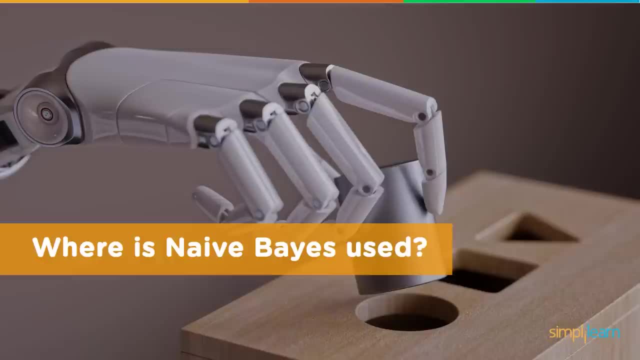 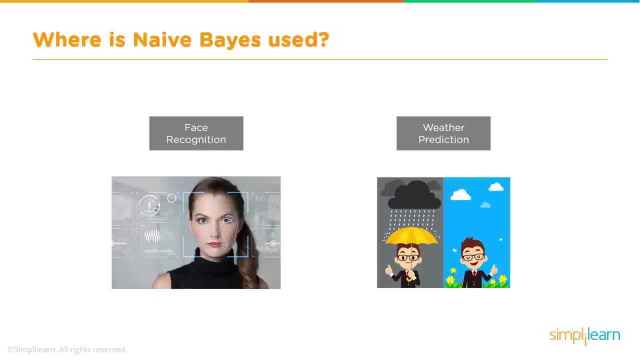 go ahead and glance into where is naive Bayes used. Let's look at some of the used scenarios for it. As a classifier, we use it in face recognition- Is this Cindy, or is it not Cindy, or whoever? Or it might be used to identify parts of the face that 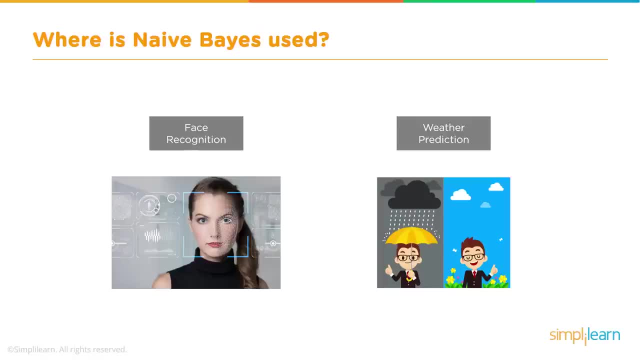 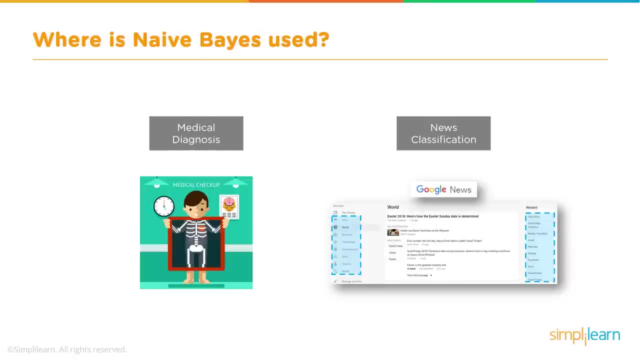 they then feed into another part of the face recognition program. This is the eye, this is the nose, this is the mouth. Weather prediction: Is it going to be rainy or sunny? Medical recognition News prediction. It's also used in medical. 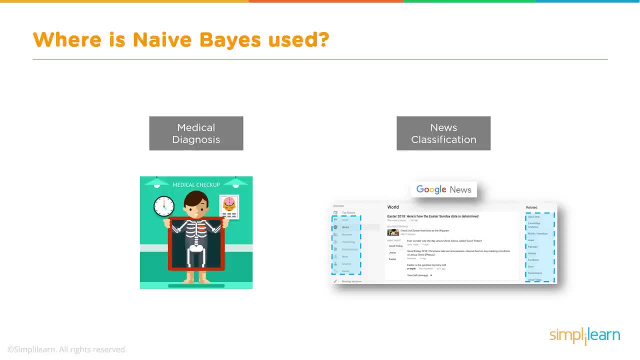 diagnosis: We might diagnose somebody as either as high risk or not as high risk for cancer or heart disease or other elements. News classification: You look at the Google News and it says, well, is this political or is this world news? or a lot of that's all done with the naive Bayes. 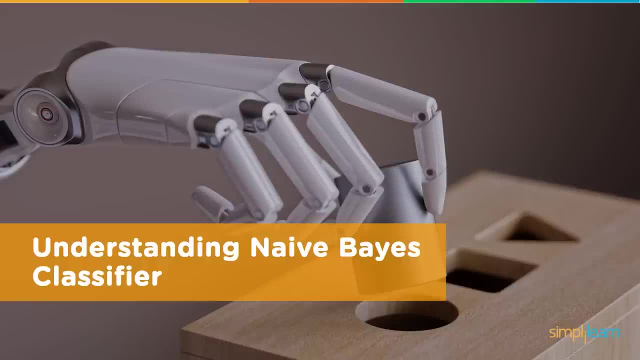 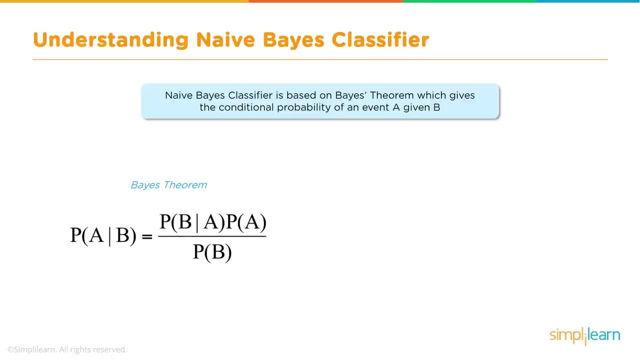 Understanding naive Bayes classifier Now. we already went through a basic understanding with the coins and the two heads and two tells and head tell, tell heads, etc. We're going to do just a quick review on that and remind you that the naive Bayes classifier is based on the Bayes theorem, which gives a conditional 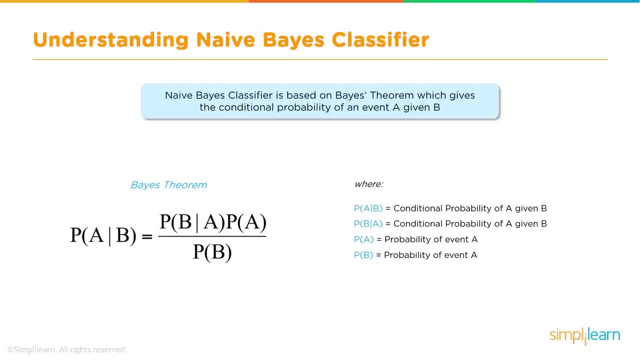 probability of event A given event B, And that's where the probability of A given B equals the probability of B given A, times probability of A over probability of B. Remember, this is an algebraic function so we can move these different entities around. We can. 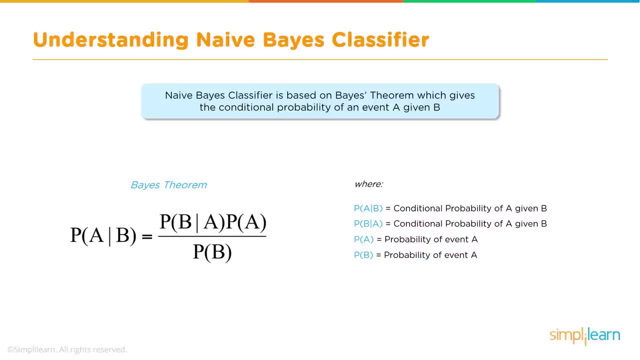 multiply by the probability of B, so it goes to the left-hand side. and then we could divide by the probability of A given B and just as easily come up with a new formula for the probability of B. To me, staring at these algebraic functions kind of gives me a slight headache. It's a lot better to see if we 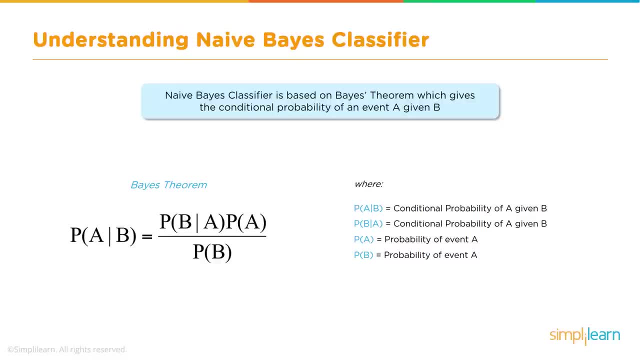 can actually understand how these things work. I'm going to show you how to do this, So let's go ahead and start applying it to some actual data so you can see what that looks like. So we're going to start with the shopping demo problem statement. 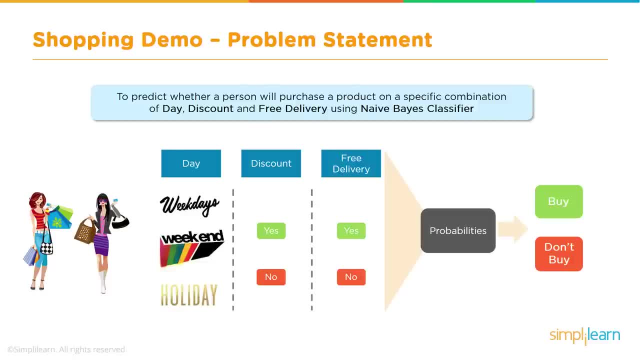 and remember, we're going to solve this first in table form, so you can see what the math looks like, and then we're going to solve it in Python, And in here we want to predict whether the person will purchase a product. Are they going to buy? 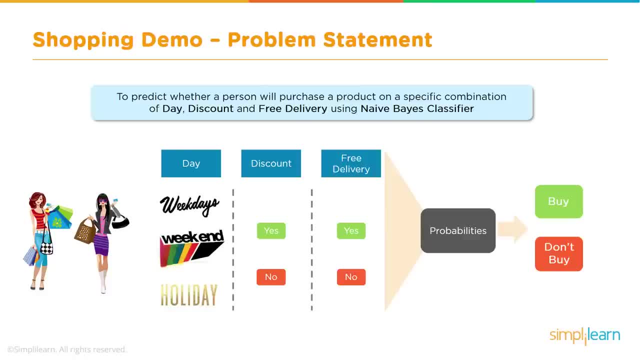 or don't buy. Very important. if you're running a business, you want to know how to maximize your profits or at least maximize the purchase of the people coming into your store, And we're going to look at a specific combination of different variables. In this case, we're going to look at the day, the discount and 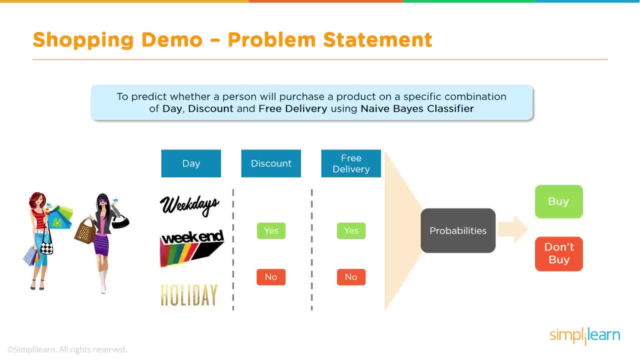 the free delivery And you can see here under the day. we want to know whether it's on the weekday. you know somebody's working, they come in after work or maybe they don't work Weekend. you can see the bright colors coming down there. 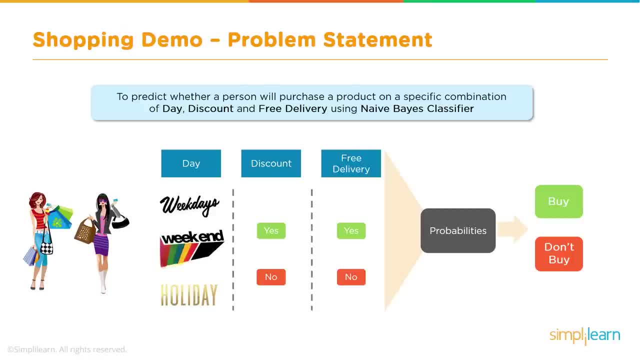 celebrating not being in work or holiday, And did we offer a discount that day, Yes or no? Did we offer free delivery that day, Yes or no? And from this we want to know whether the person is going to buy based on these traits, so we can maximize. 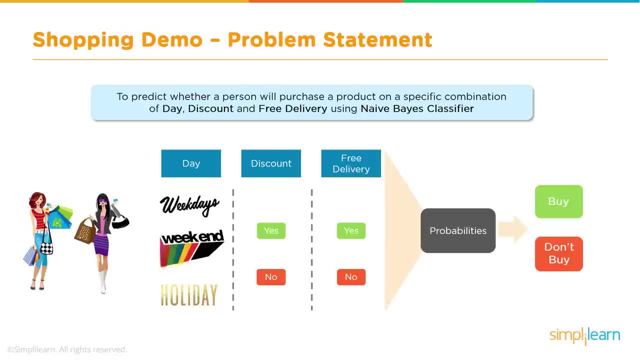 them and find out the best system for getting somebody to come in and buy a discount and purchase our goods and products from our store. Now, having a nice visual is great, but we do need to dig into the data. So let's go ahead and 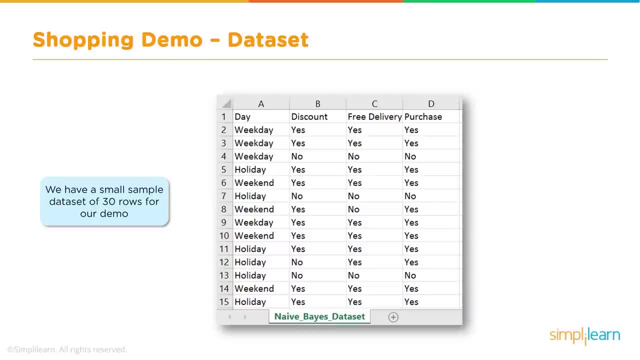 take a look at the data set. We have a small sample data set of 30 rows. We're showing you the first 15 of those rows for this demo. Now the actual data file you can request, just type in below under the comments on the YouTube video and. 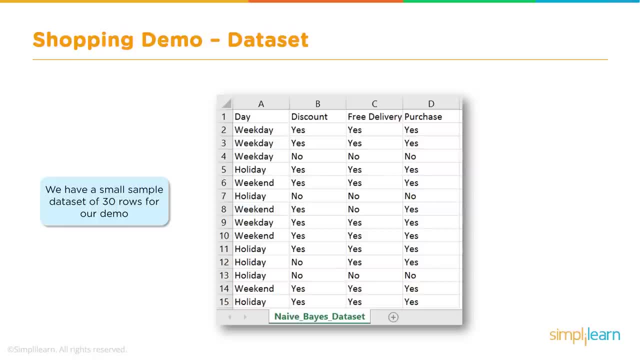 we'll send you some more information and send you that file. As you can see here, the file is very simple: columns and rows. We have the day, the discount, the free delivery, and did the person purchase or not? And then we have under the day, 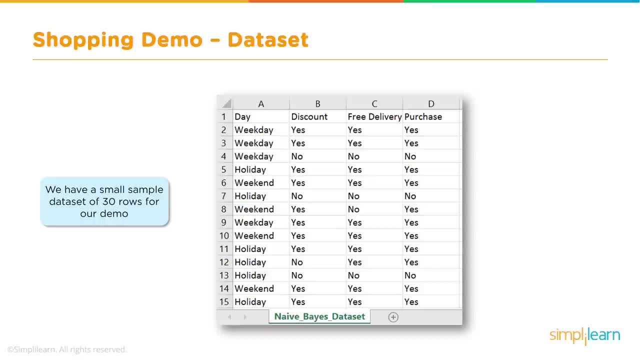 whether it was a weekday, a holiday, was it the weekend? This is a pretty simple set of data and long before computers, people used to look at this data and calculate this all by hand. So let's go ahead and walk through this and see what. 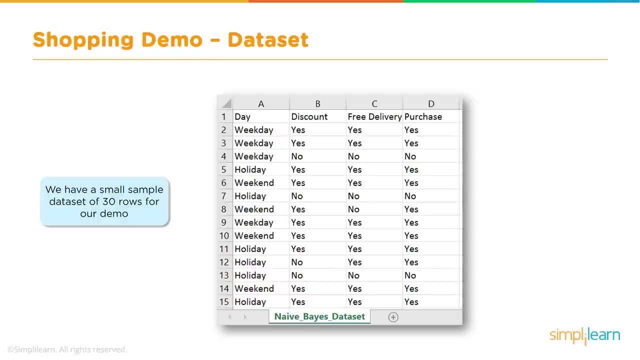 that looks like when we put that into tables. Also note: in today's world we're not usually looking at three different variables in 30 rows. Nowadays, because we're able to collect data so much, we're usually looking at 27,- 30 variables. 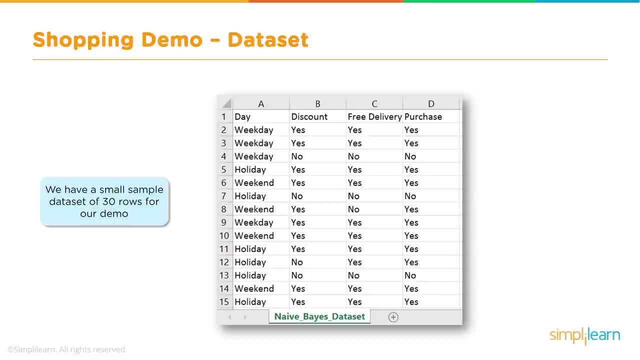 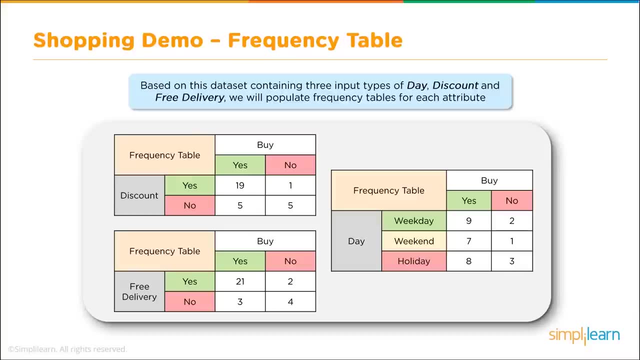 across hundreds of rows. The first thing we want to do is we're going to take this data and, based on the data set containing our three inputs- day, discount and free delivery- we're gonna go ahead and populate that to frequency tables for each attribute. So we want to know, if they had a discount, how many people buy. 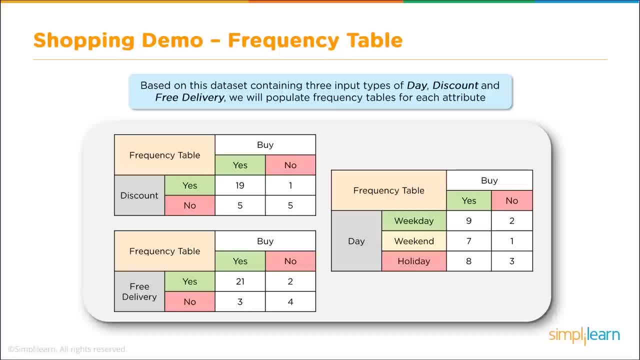 and did not buy. did they have a discount, yes or no? do we have a free delivery, yes or no? on those days, how many people made a purchase, how many people didn't? and the same with the three days of the week. Was it a weekday, a weekend, a holiday? 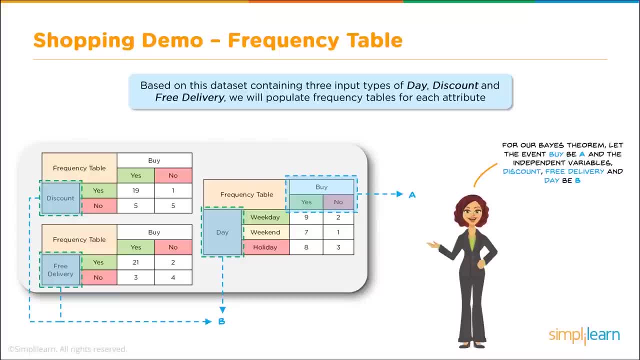 and did they buy, yes or no? As we dig in deeper to this table for our Bayes theorem, let the event buy be A. Now remember we looked at the coins. I said we really want to know what the outcome is. did the person buy or not? and that's. 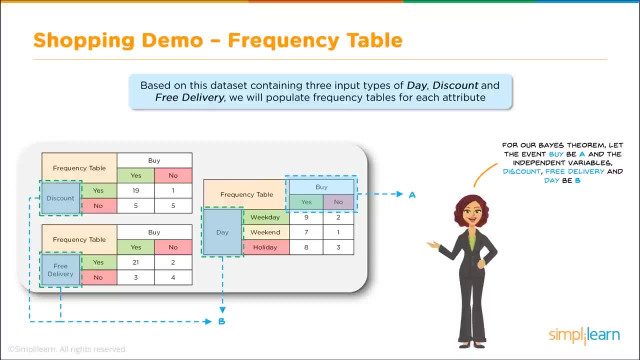 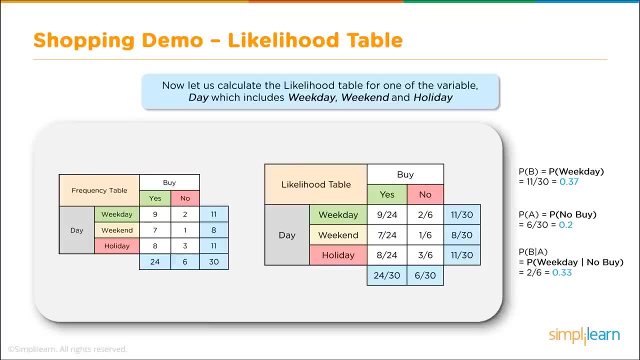 usually event A is what you're looking for And the independent variables discount, free delivery and day be B, So we'll call that probability of B. Now let us calculate the likelihood table for one of the variables. Let's start with day, which includes weekday, weekend and holiday, And let us start by summing all. 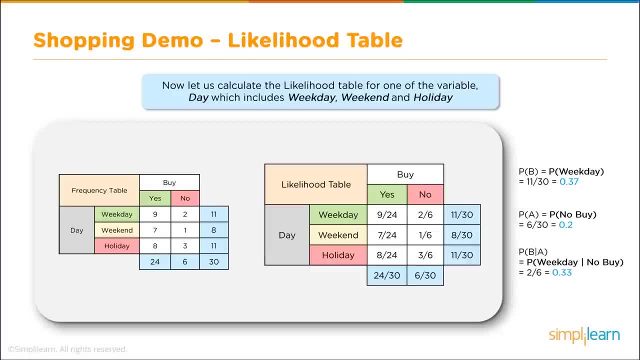 of our rows. So we have the weekday row and out of the weekdays there's nine plus two, so it's eleven weekdays. There's eight weekend days and eleven holidays. That's a lot of holidays. And then we want to sum up the total number of days. 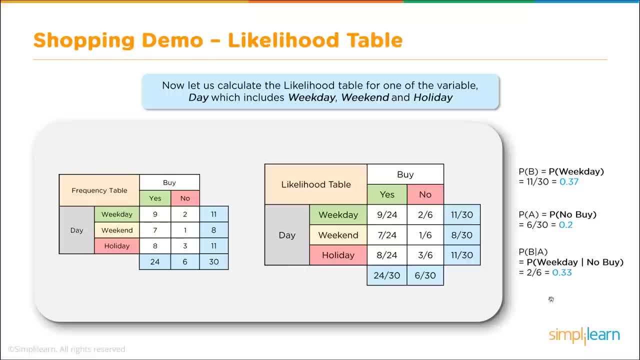 So we're looking at a total of 30 days. Let's start pulling some information from our chart and see where that takes us. And when we fill in the chart on the right, you can see that nine out of 24 purchases are made on the weekday seven. 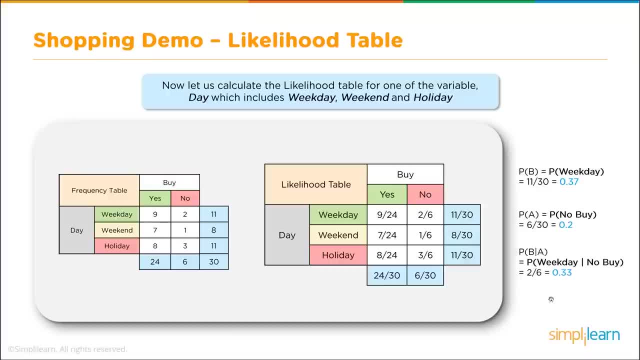 out of 24 purchases on the weekend and eight out of 24 purchases on a holiday. And out of all the people who come in, twenty-four out of 30 purchase. You can also see how many people do not purchase On the weekday. it's two out of six didn't purchase, and so on, and so on. 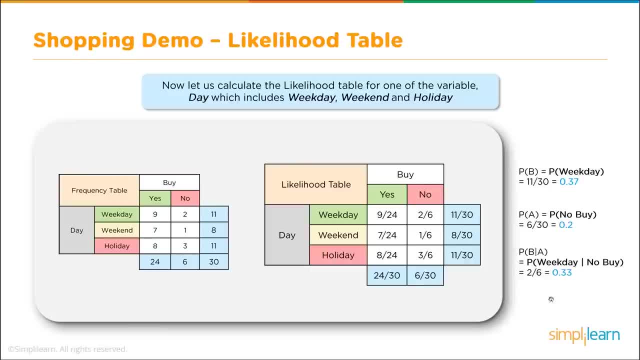 We can also look at the totals and you'll see. on the right we put together some of the formulas. the probability of making a purchase on the weekend comes out at 11 out of 30.. So out of the 30 people who came into the store throughout the 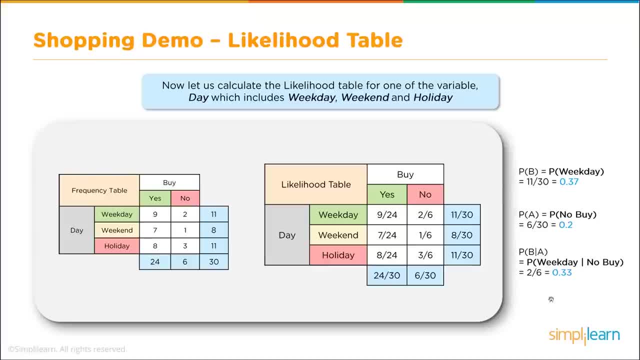 weekend, weekday and holiday. eleven of those purchases were made on the weekday, And then you can also see the of them not making a purchase, and this is done for doesn't matter which day of the week. so we call that probability of no buy would be 6 over 30 or 0.2, so there's a 20% chance that they're. 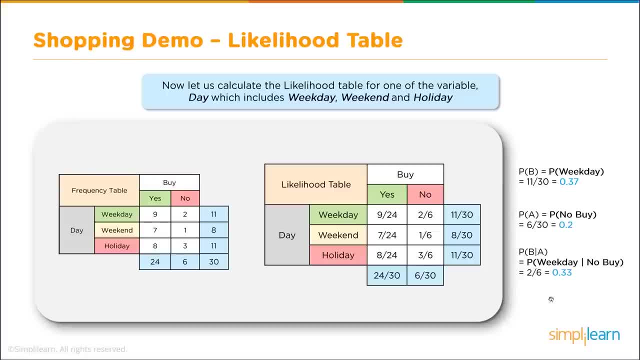 not going to make a purchase, no matter what day of the week it is. and finally, we look at the probability of BFA. in this case, we're gonna look at the probability of the weekday and not buying. two of the no buys were done out of the weekend out of the six people who did not make purchases. 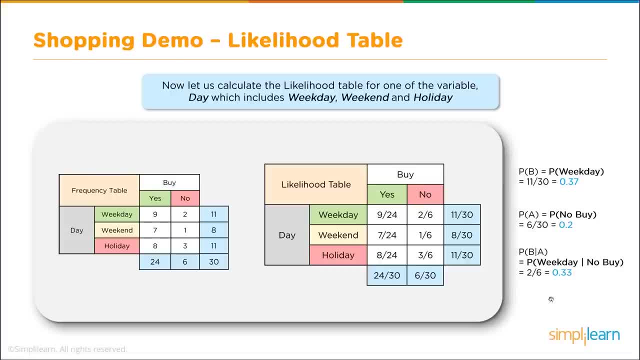 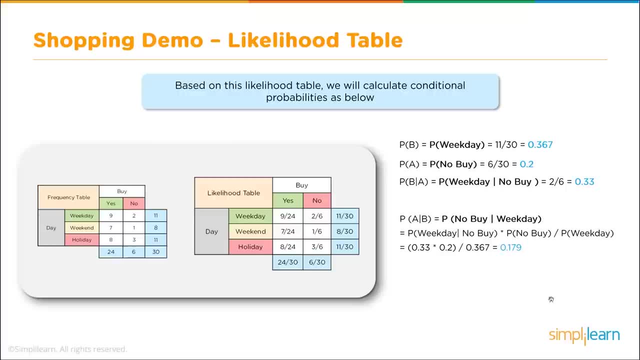 so when we look at that probability of the weekday without a purchase is going to be 0.33 or 33%, let's take a look at this, at different probabilities, and, based on this likelihood table, let's go ahead and calculate conditional probabilities as below the first three. we just did the probability. 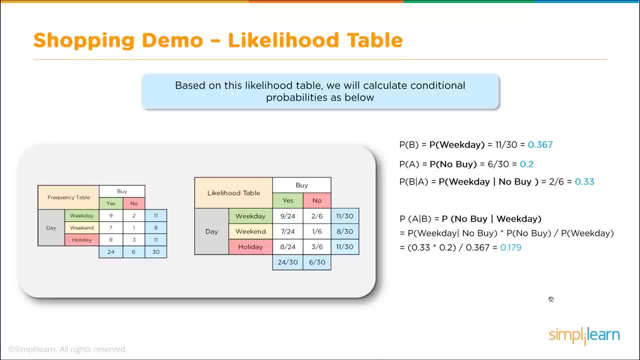 of making a purchase on the weekday is 11 out of 30, or roughly 36 or 37 percent- 0.367. the probability of not making a purchase at all, doesn't matter what day of the week, is roughly 0.2 or 20 percent, and the probability of a weekday no purchase is roughly 2 out of 6. so 2 out of 6 of. 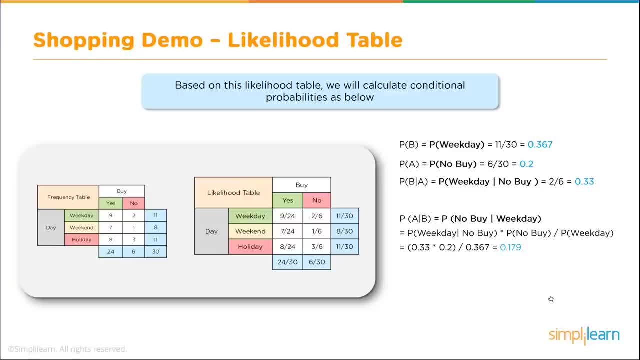 our no purchases were made on the weekday. and then, finally, we take our P of a- b. if you look, we've kept the symbols up there. we got P of probability B: probability of a. probability of b if a. we should remember that the probability of a if b is equal to the first one times the. 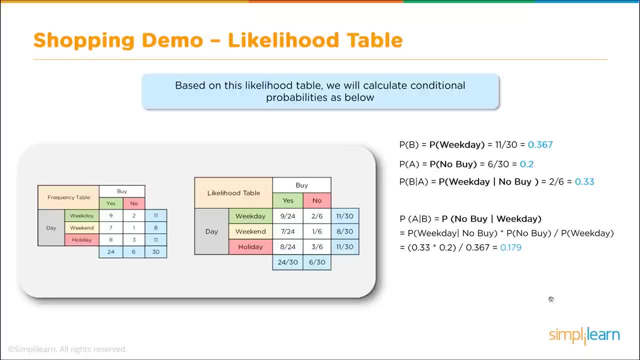 probability of no pour buys over the probability of the weekday. So we could calculate it both off the table we created. We can also calculate this by the formula and we get the 0.367, which equals or 0.33 times 0.2 over 0.367, which equals 0.179. 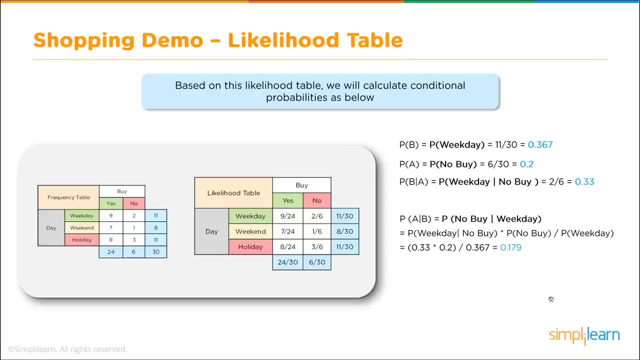 or roughly 17 to 18 percent, And that'd be the probability of no purchase done on the weekday. And this is important because we can look at this and say, as the probability of buying on the weekday is more than the probability of not buying on the weekday, we can conclude that 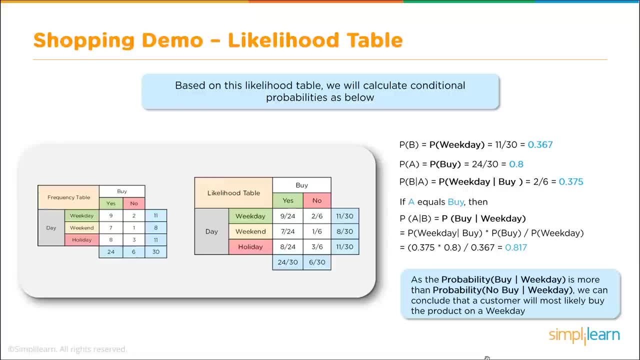 customers will most likely buy the product on a weekday. Now we've kept our chart simple and we're only looking at one aspect, So you should be able to look at the table and come up with the same information or the same conclusion. That should be kind of intuitive at this point. Next, we can take: 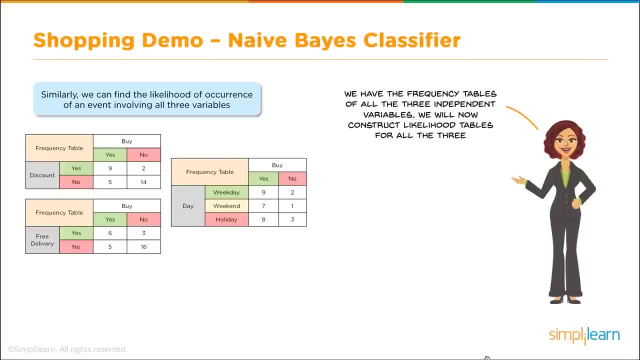 the same setup. We have the frequency tables of all three independent variables. Now we can construct the likelihood tables for all three of the variables we're working with. We can take our probability tables for all three of the variables we're working with. We can take our 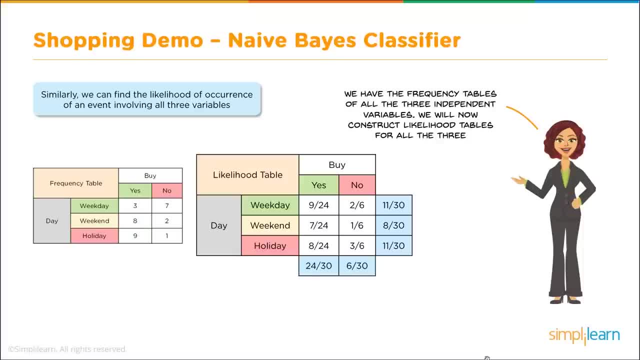 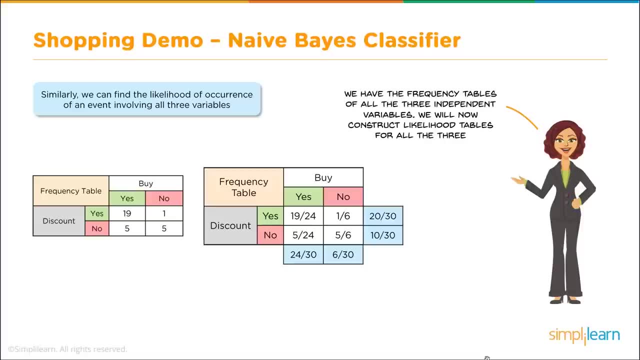 day, like we did before. We have weekday, weekend and holiday. We filled in this table And then we can come in and also do that for the discount- Yes or no? Did they buy, Yes or no? And we fill in that full table. So now we have our probabilities for a discount and whether the discount leads to. 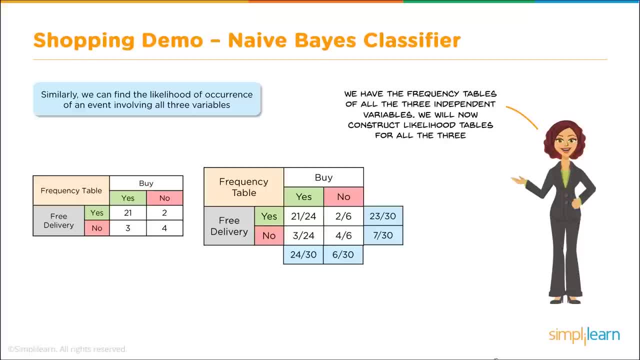 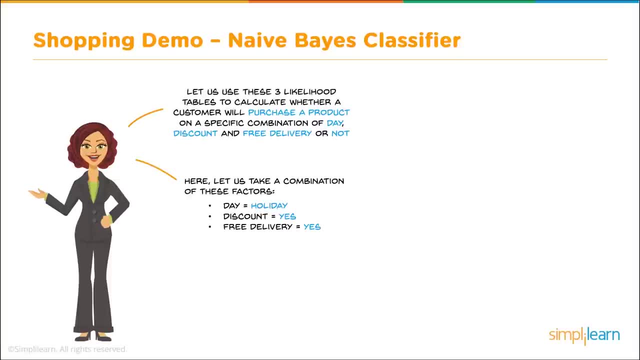 a purchase or not? And the probability for free delivery. Does that lead to a purchase or not? And this is where it starts getting really exciting. Let us use these three likelihood tables to calculate whether a customer will purchase a product on a specific combination of day discount and free delivery or not purchase. Here let us take a combination. 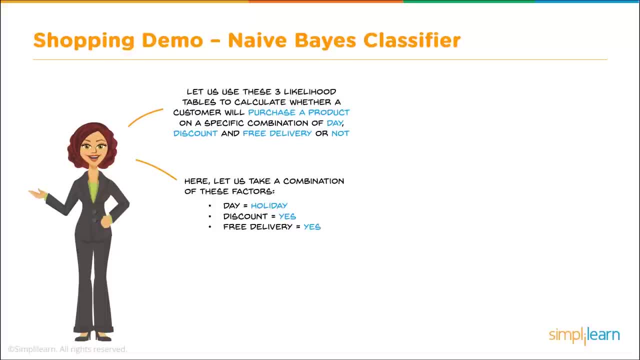 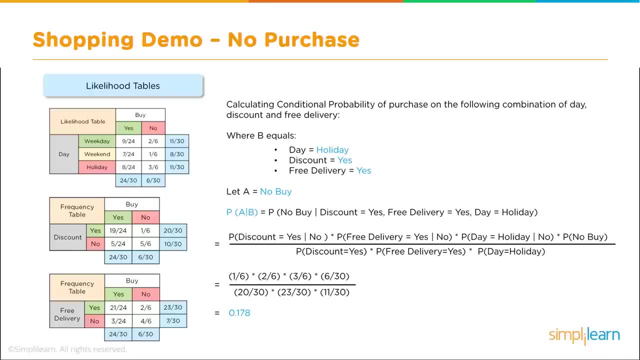 of these factors: Day equals holiday. Discount equals yes. Free delivery equals yes. Let's dig deeper into the math and actually see what this looks like, And we're going to start with looking for the probability of them not purchasing on the following combinations of days. We're actually 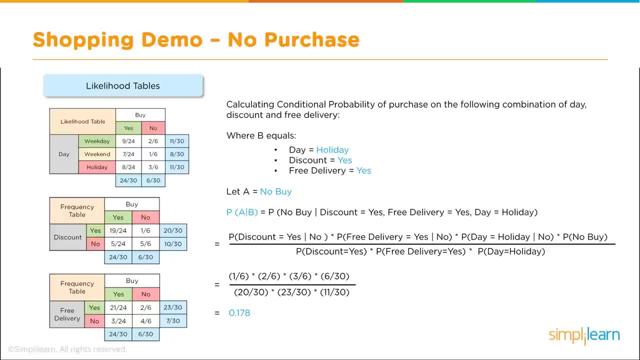 looking for the probability of A- equal no buy, no purchase- And our probability of B. we're going to set equal to: is it a holiday or a free delivery? And we're going to set equal to: is it a holiday? Did they get a discount? Yes, And was it a free delivery? Yes. Before we go further, let's 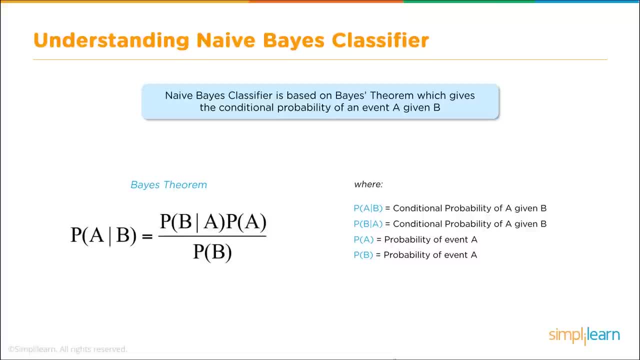 look at the original equation: The probability of A if B equals the probability of B, given the condition A and the probability times the probability of A over the probability of B occurring. Now this is basic algebra, so we can multiply this information together. So when you 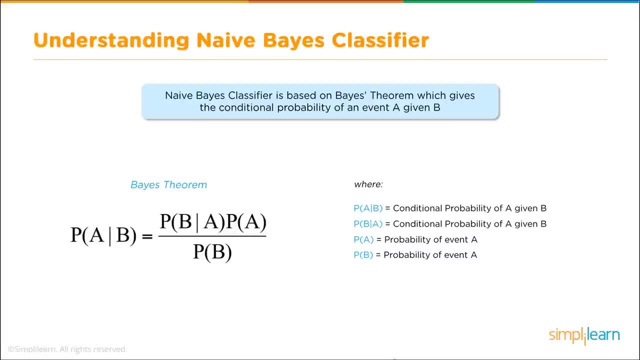 see the probability of A given B. in this case the condition is B, C and D, or the three different variables we're looking at, And when you see the probability of B, that would be the conditions. We're actually going to multiply those three separate conditions out. Probability of you'll see. 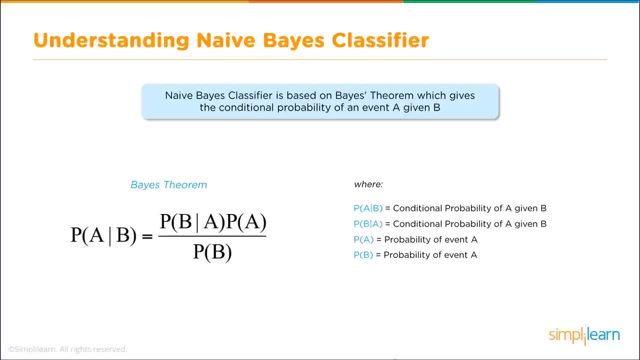 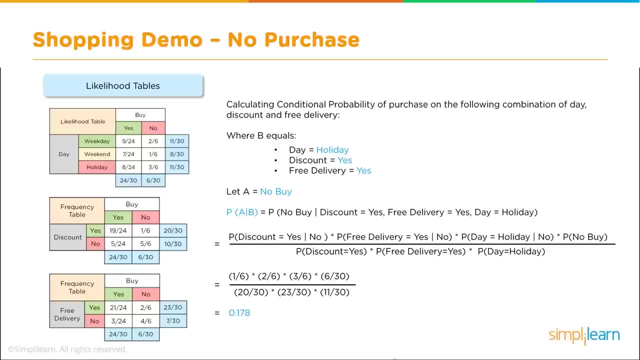 that in just a second in the formula times the full probability of A over the full probability of B. So here we are back to this and we're going to have let A equal no purchase And we're looking for the probability of B on the condition A, where A sets for three different things. Remember that. 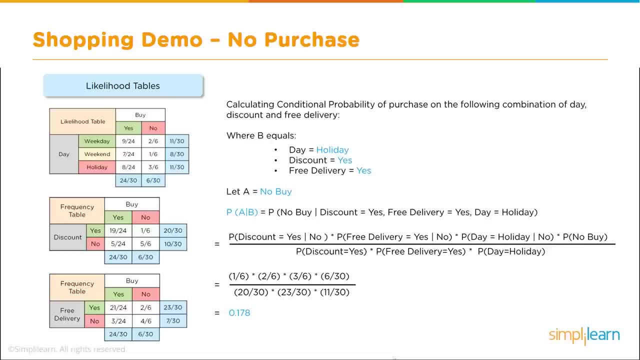 equals the probability of A, given the condition A, where the probability of A equals no buy, And we're condition B, and in this case we just multiply those three different variables together. So we have the probability of the discount times, the probability of free delivery times, 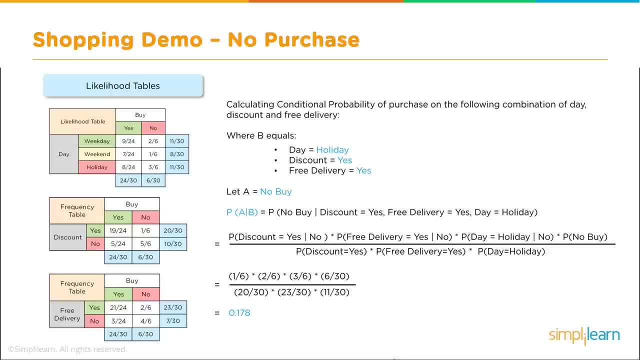 the probability is the day equal holiday. Those are our three variables of the probability of A. if B, and then that is going to be multiplied by the probability of them not making a purchase, And then we want to divide that by the total probabilities and they're multiplied together. 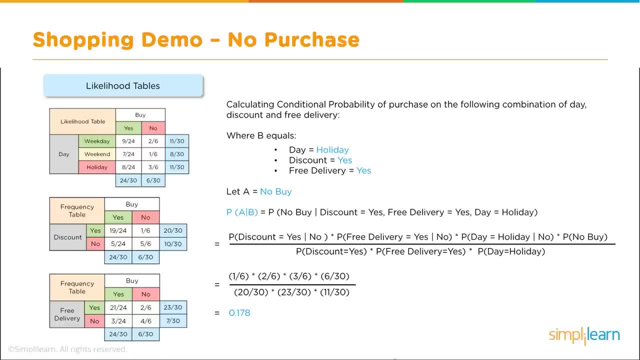 So we have the probability of a discount, the probability of a free delivery and the probability of it being on a holiday. When we plug those numbers in, we see that one out of six were no purchase on a discounted day, two out of six were a no purchase on a free delivery day and three out of six 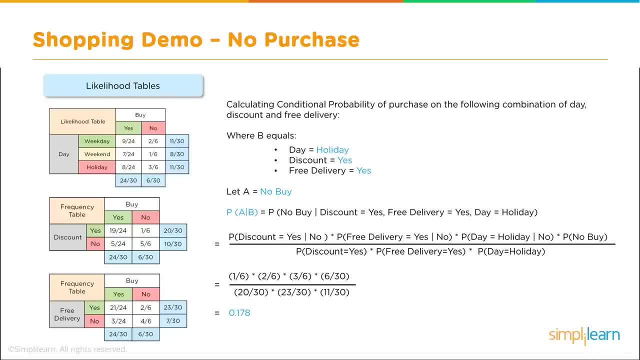 were a no purchase on a holiday. Those are our three probabilities of A if B multiplied out. and then that has to be multiplied by the probability of a no purchase. And remember the probability of a no buy is across all the numbers. So that's where we get the six out of 30.. 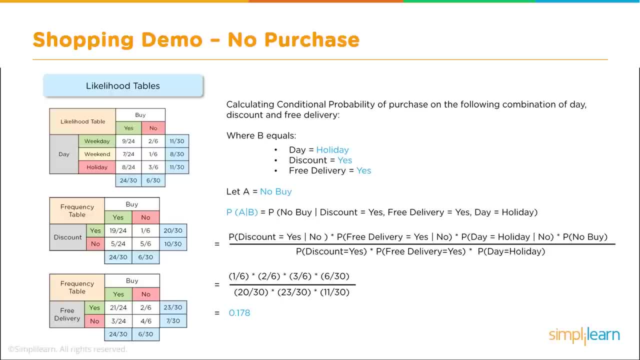 We divide that out by the probability of each category over the total number, So we get the 20 out of 30 had a discount, 23 out of 30 had a yes for free delivery and 11 out of 30 were on a holiday. 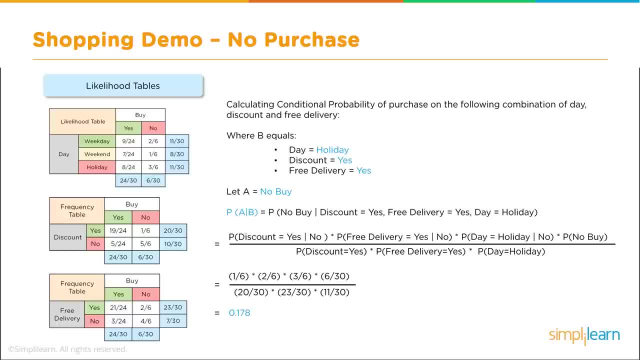 We plug all those numbers in, we get .178.. So in our probability math we have a .178. if it's a no buy for a holiday, a discount and a free delivery, Let's turn that around and see what that looks like. if we have a purchase, 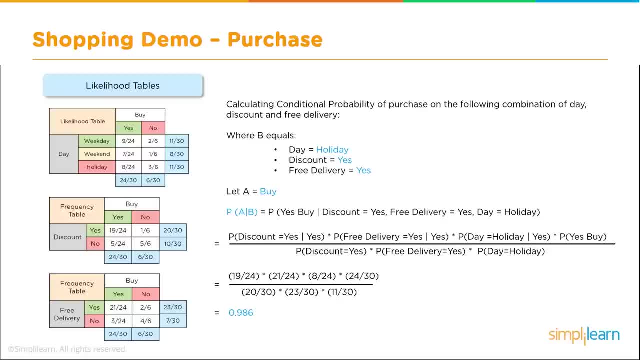 I promise this is the last page of math before we dig into the Python script. So here we're, calculating the probability of the purchase using the same math we did to find out if they didn't buy. Now we want to know if they did buy. 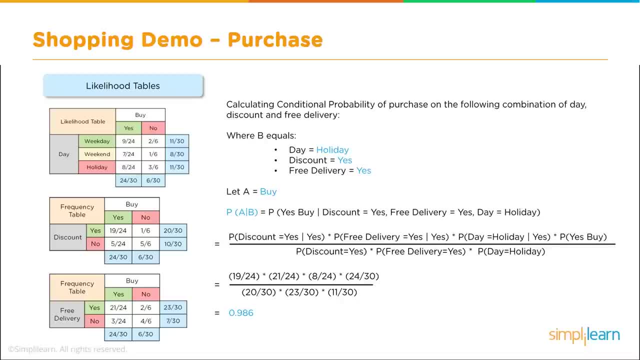 And again we're going to go by the day: equals a holiday discount equals yes, free delivery equals yes. and let A equal buy. Now, right about now, you might be asking: why are we doing both calculations? Why would we want to know the no buys and buys for the same data going in? 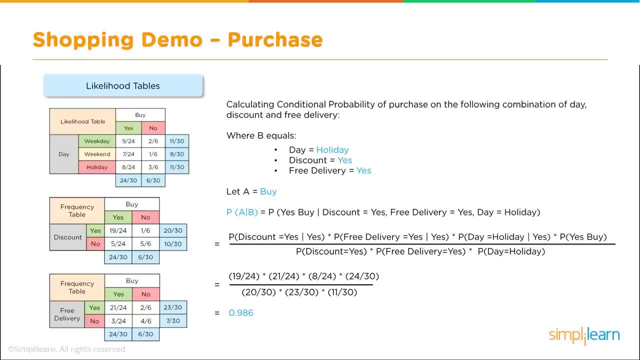 Well, we're going to show you that in just a moment. but we have to have both of those pieces of information so that we can figure it out as a percentage as opposed to a probability equation. And we'll get to that normalization here in just a moment. 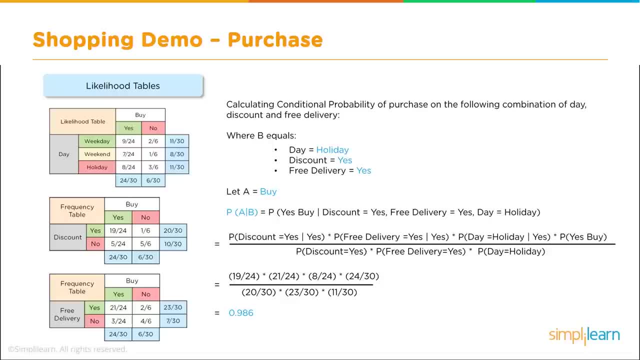 Let's go ahead and walk through this calculation And, as you can see here, the probability of A on the condition of B, B being all three categories, did we have a discount with a purchase? do we have a free delivery with a purchase? and is a day equal to holiday? And when we plug this all into that formula and multiply it all up, we get .178.. So that's the probability of A on the condition of B, B being all three categories. did we have a discount with a purchase? did we have a free delivery with a purchase? and is a day. 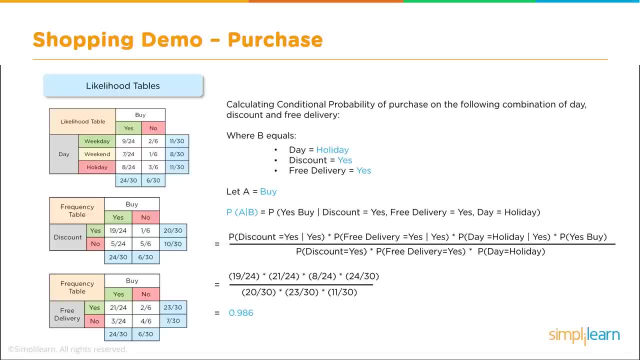 equal to holiday, We get our probability of a discount, probability of a free delivery, probability of the day being a holiday times the overall probability of it being a purchase, divided by again multiplying the three variables out, the full probability of there being a discount, the full probability. 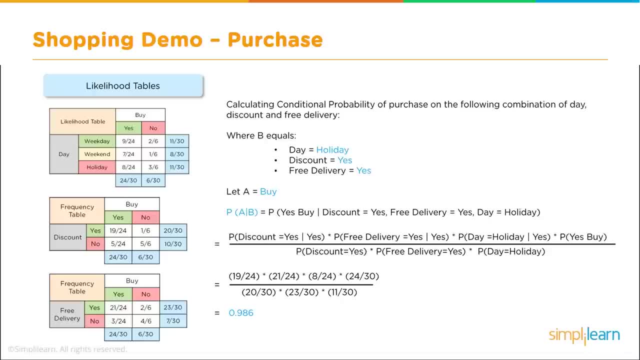 of being a free delivery and the full probability of there being a day equal holiday, And that's where we get this: 19 over 24 times 21 over 24 times, 8 over 24 times the P of A 24 over 30.. 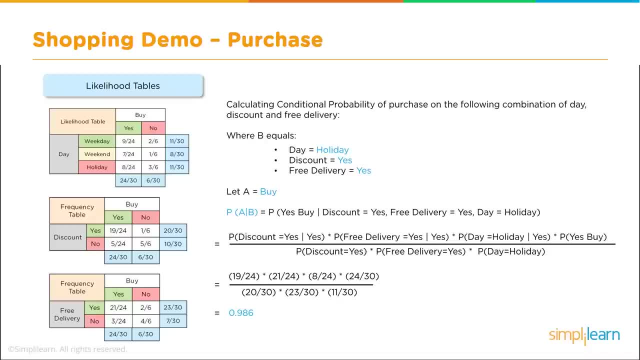 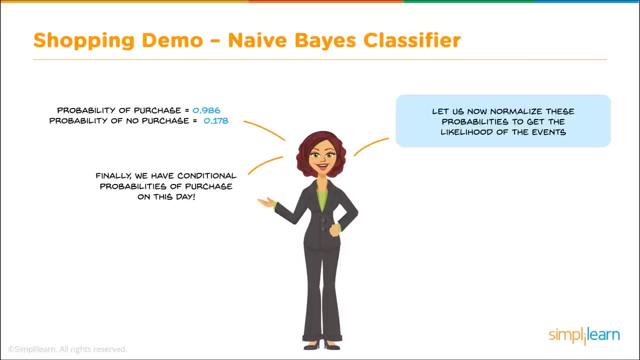 A day equal to a discount. probability of a free delivery. probability of a free delivery times the day being a holiday. probability of a free delivery. probability of a free delivery times the day being a holiday. and that gives us our .986.. 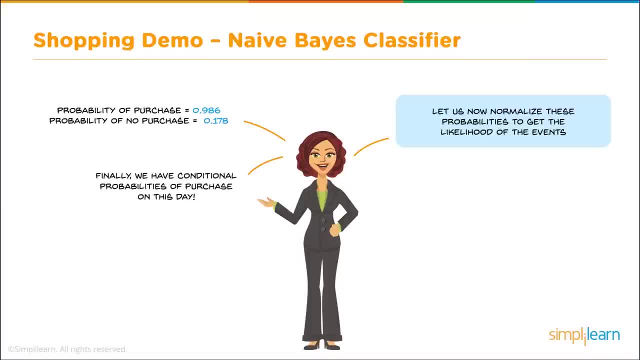 So let's go ahead and go over them. we have a probability of a purchase equals .986,. we have a probability of no purchase equals .178.. So, finally, we have a conditional probability this day. Let us take that we're going to normalize it and we're going to take these. 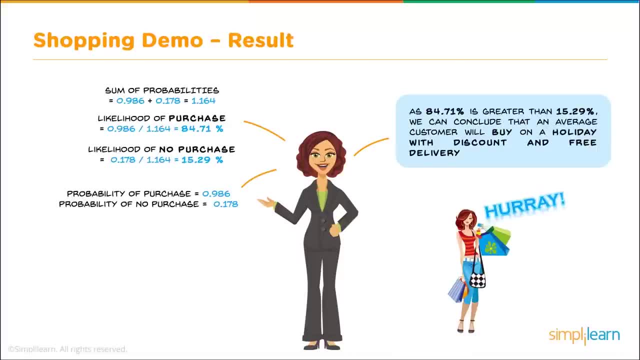 probabilities and turn them into percentages. This is simply done by taking the sum of probabilities, which equals 0.98686 plus 0.178, and that equals the 1.164.. If we divide each probability by the sum, we get the percentage, And so the likelihood of a purchase is 84.71%. 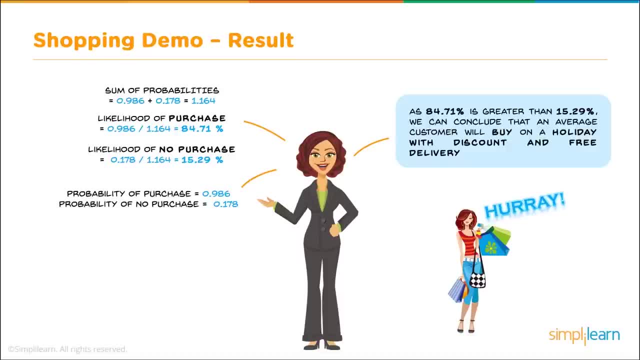 and the likelihood of no purchase is 15.29%, given these three different variables. So if it's on a holiday, if it's with a discount and has free delivery, then there's an 84.71% chance that the customer is going to come in and make a purchase. Hooray, They purchased our stuff. 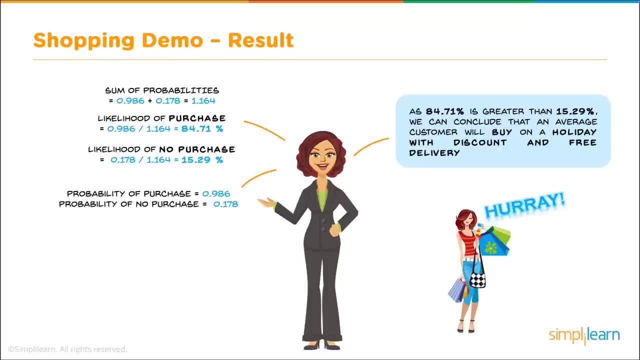 We're making money. If you're owning a shop, that's like is the bottom line is you want to make some money so you can keep your shop open and have a living. Now I promised you that we were going to be finishing up the math here with a few pages, So we're going to move on and we're 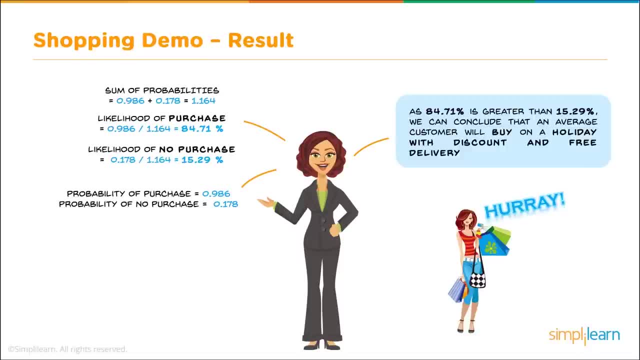 going to do two more. We're going to do two more. We're going to do two more. We're going to do two steps. The first step is: I want you to understand why you want to use the Naive Bayes. What are the advantages of Naive Bayes? And then, once we understand those advantages, 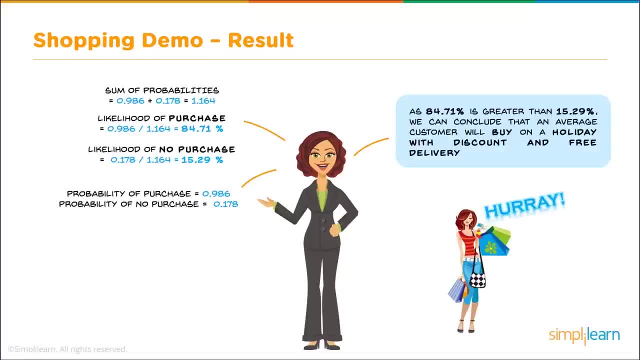 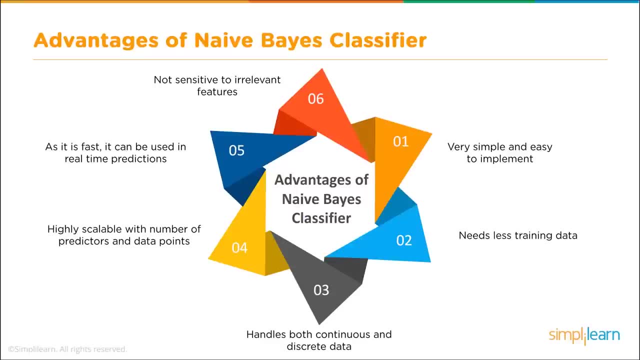 we'll just look at that briefly. then we're going to dive in and do some Python coding. Advantages of Naive Bayes Classifier. So let's take a look at the six advantages of the Naive Bayes Classifier and we're going to walk around this lovely wheel. It looks like. 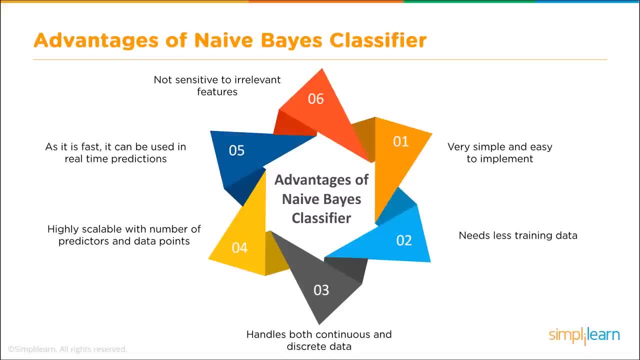 an origami folded paper. The first one is very simple and easy to implement. Certainly you could walk through the tables and do this by hand. You got to be a little careful because the notations can get confusing. You have all these different probabilities and I certainly 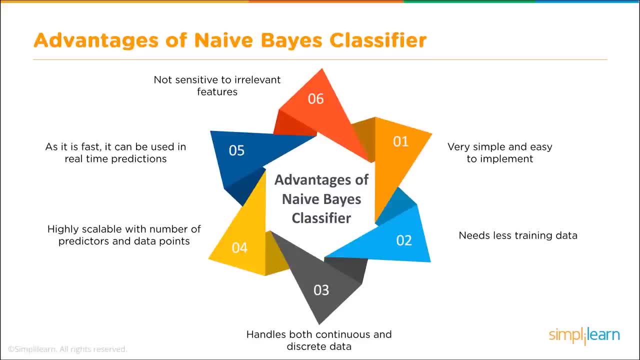 mess those up as I put them on. you know, is it on the top or the bottom? You got to really pay close attention to that. When you put it into Python, it's really nice because you don't have to worry about any of that. You let the Python handle that, the Python module. But understanding. 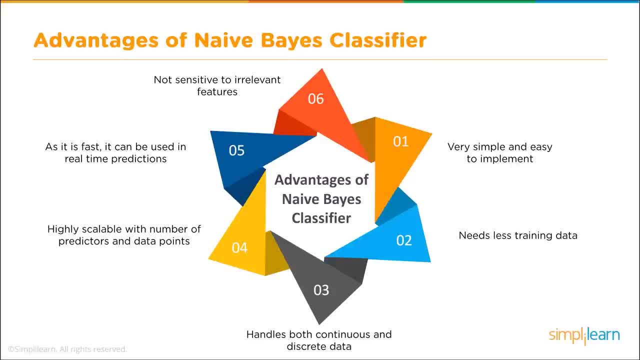 it. you can put it on a table and you can easily see how it works. and it's a simple algebraic function. It needs less training data. So if you have smaller amounts of data, this is a great powerful tool for that Handles both continuous and discrete data. It's highly scalable. 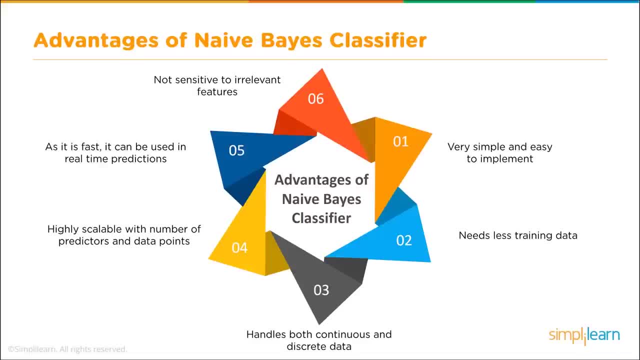 with number of predictors and data points. So, as you can see, you just keep multiplying different probabilities in there and you can cover not just three different variables or sets. You can now expand this to even more categories. Number five: it's fast, It can be used in real-time. 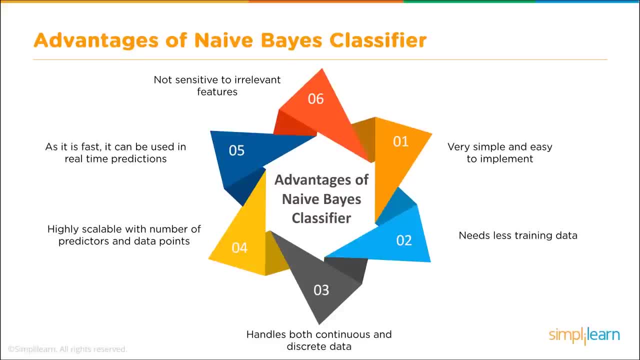 predictions. This is so important. This is why it's used in a lot of our predictions on online shopping carts, referrals, spam filters- is there's no time delay as it has to go through and figure out a neural network or one of the other. 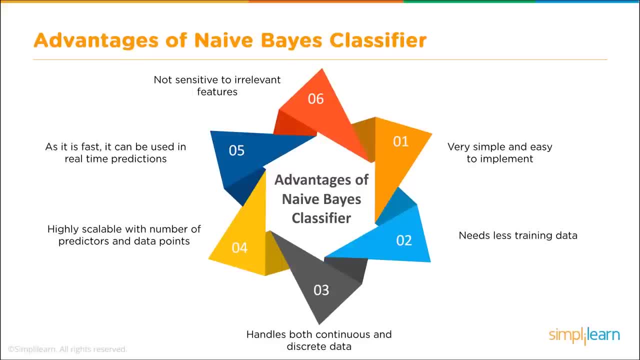 many setups where you're doing classification, And certainly there's a lot of other tools out there in the machine learning that can handle these, but most of them are not as fast as a naive base. And then, finally, it's not sensitive to irrelevant features, So it picks up on your 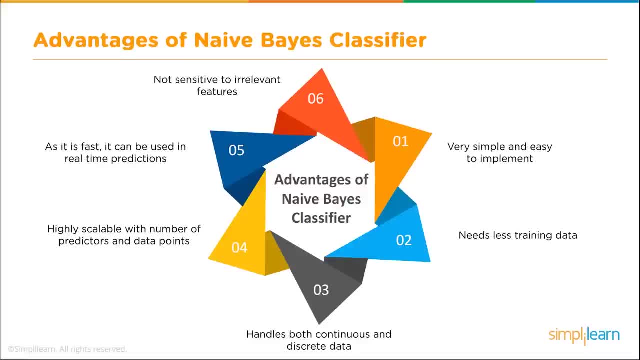 different probabilities, and if you're short on data on one probability, you can kind of it automatically adjust for that. Those formulas are very automatic, and so you can still get a very solid predictability even if you're missing data or you have overlapping data for two completely. 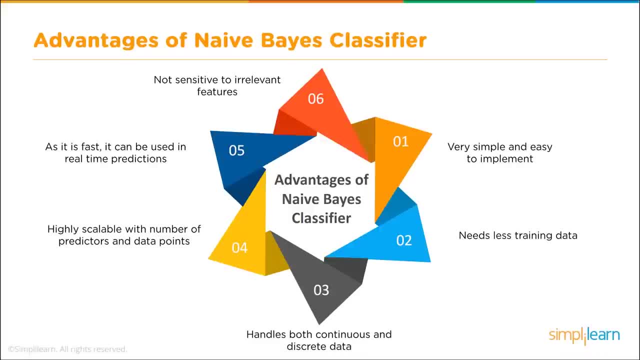 different areas. We see that a lot in doing census and studying of people and habits, where they might have one study that covers one aspect, another one that overlaps, and because the two overlap they can then predict the unknowns for the group that they haven't done the second study on or vice. 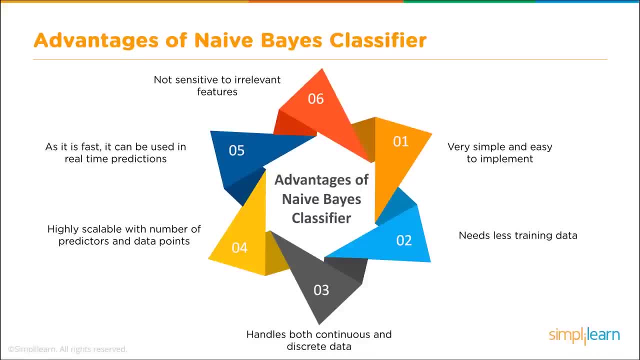 versa. So it's very powerful in that it is not sensitive to the irrelevant features and in fact, you can use it to help predict features that aren't even in there. So now we're down to my favorite part: We're going to roll up our sleeves and do some actual 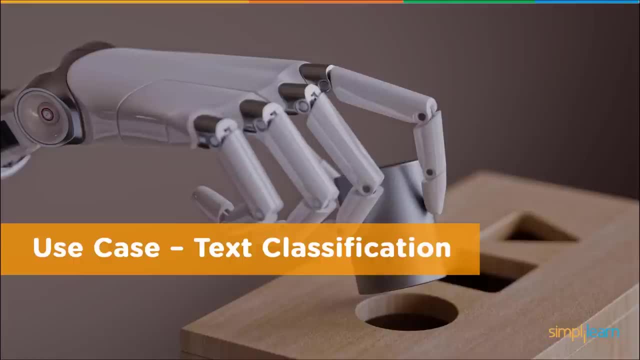 programming. We're going to do the use case text classification Now I would challenge you to go back and send us a note on the notes below underneath the video and request the data for the shopping cart. So you can plug that into Python code and do that on your own time, so you 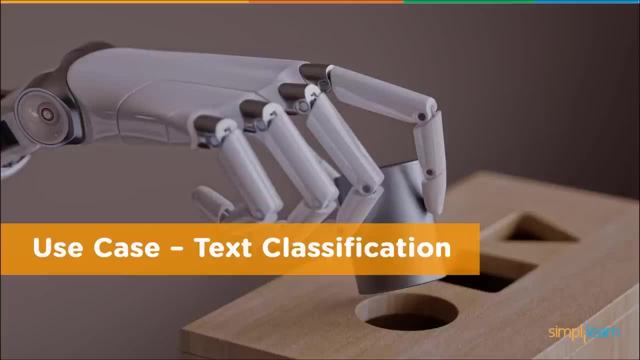 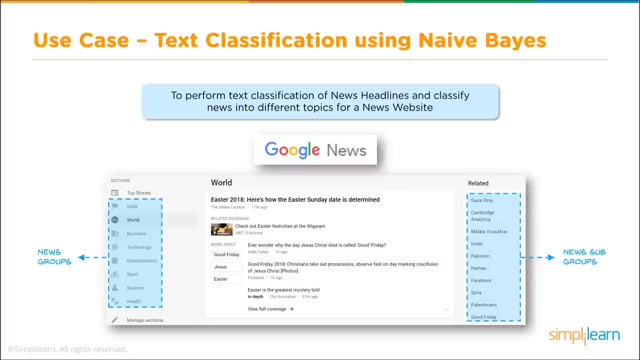 can walk through it, since we walked through all the information on it. But we're going to do a Python code doing text classification- very popular for doing the naive base. So we're going to use our new tool to perform a text classification of news headlines and classify. 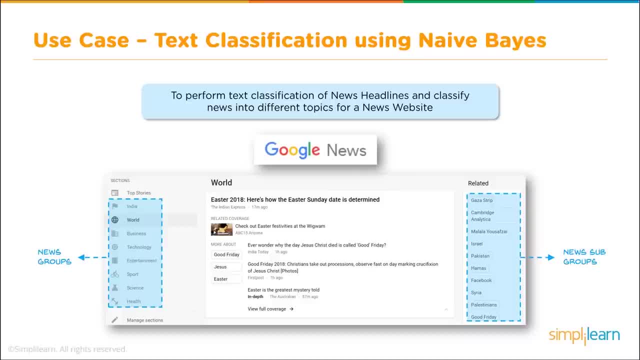 news into different topics for a news website. As you can see here we have a nice image of the Google News and then related on the right subgroups. I'm not sure where they actually pulled the actual data we're going to use from. It's one of the standard sets, but certainly this. 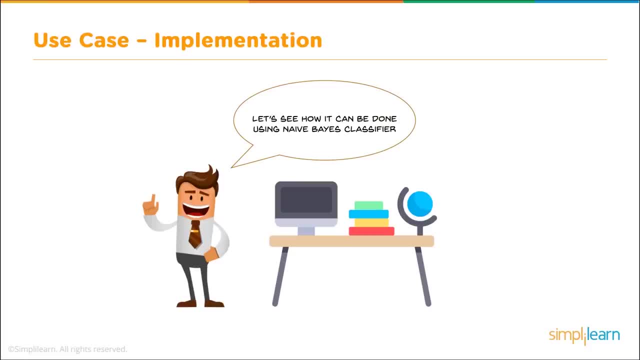 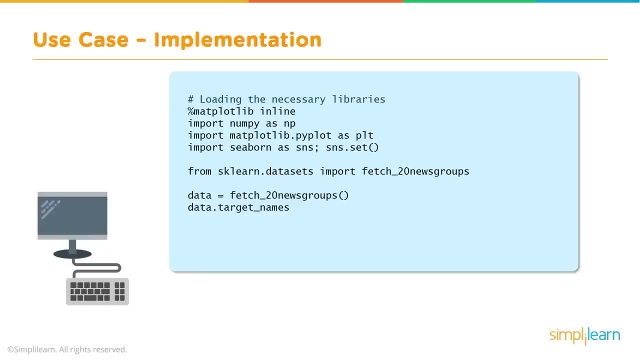 can be used on any of our news headlines and classification. So let's see how it can be done using the naive base classifier. Now we're at my favorite part. We're actually going to write some Python script, roll up our sleeves and we're going to start by doing our imports. These are: 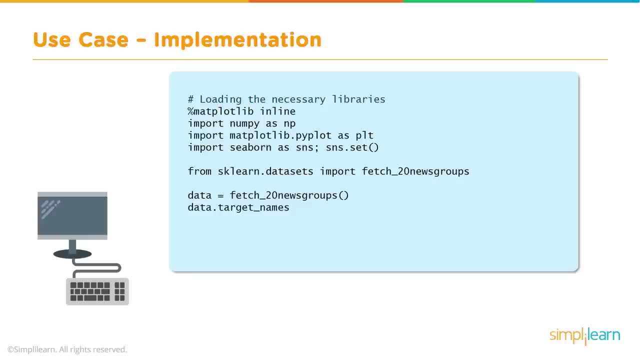 very basic imports, including our news group, And we'll take a quick glance at the target names. Then we're going to go ahead and start training our data set and putting it together. We'll put together a nice graph, because it's always good to have a graph to show what's going on. And once we've 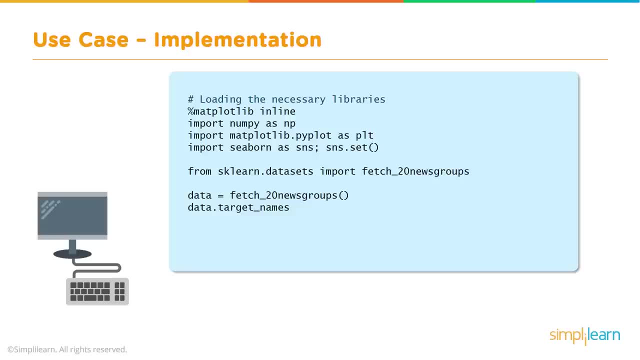 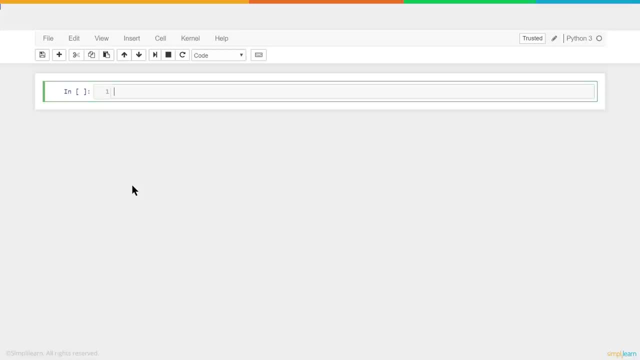 trained it and we've shown you a graph of what's going on. then we're going to explore how to use it and see what that looks like. Now I'm going to open up my favorite editor or inline editor, for whatever your editor that you like, whatever interface IDE you want. This just happens to be. 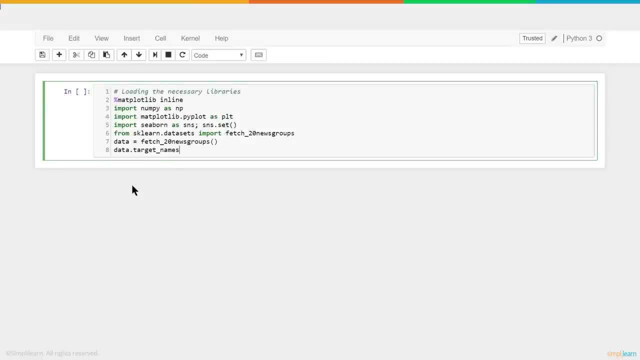 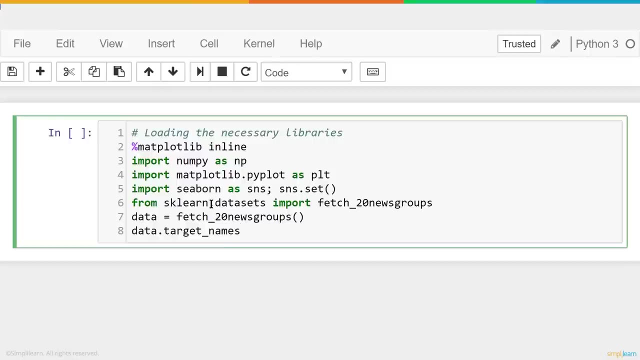 the Anaconda Jupyter notebook And I'm going to paste that first piece of code in here so we can walk through it. Let's make it a little bigger on the screen so you have a nice view of what's going on. And we're using Python 3, in this case 3.5. So this would work in any of your 3x, If you have. 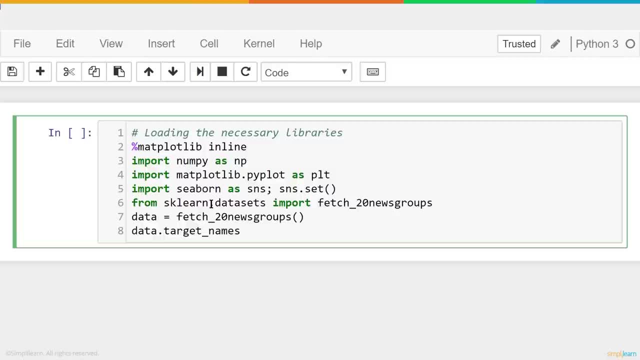 it set up correctly, it should also work in a lot of the 2x. You just have to make sure all of the versions of the modules match your Python version And in here you'll notice the first line is your percentage matplotlibrary inline. Now three of these lines of code are: 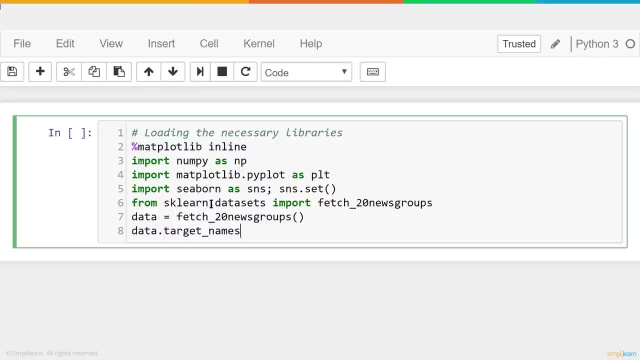 all about plotting the graph. This one lets the notebook notes- and this is the inline setup- that we want the graphs to show up on this page. Without it, in a notebook like this, which is an explorer interface, it won't show up. Now, a lot of IDEs don't require that, A lot of 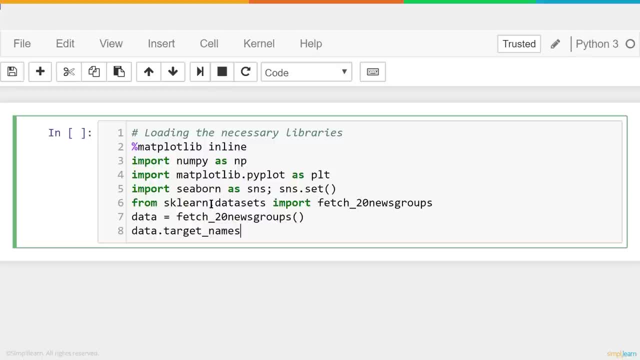 them, like if I'm working on one of my other setups, it just has a pop-up and the graph pops up on there. So you have a very nice view of what's going on And you can see that it's all about plotting the graph. But for this we want the matplotlibrary inline And then we're 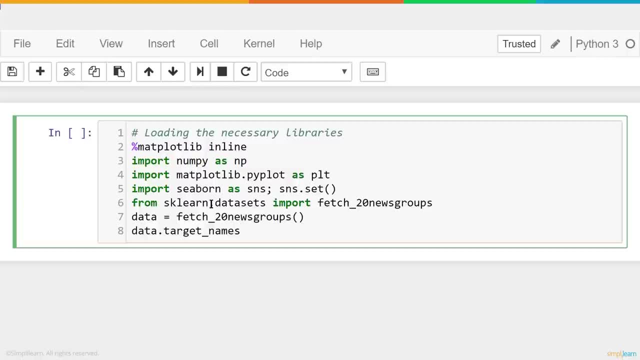 going to import numpy as np. That's number Python, which has a lot of different formulas in it that we use for both of our sklearn module And we also use it for any of the upper math functions in Python And it's very common to see that as np, numpy as np. The next two lines are all about our. 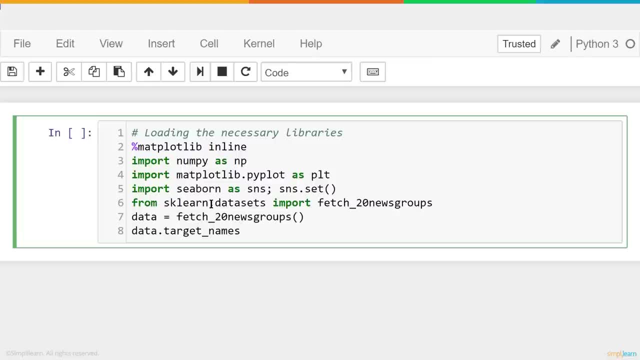 graphing. Remember, I said three of these were about graphing. Well, we need our matplotlibrarypyplot and you'll see that plt is a very common setup, as is the sns and just like the np, And we're going to import seaborn as sns and we're going to do the snsset. Now, seaborn sits on top of pyplot and it. 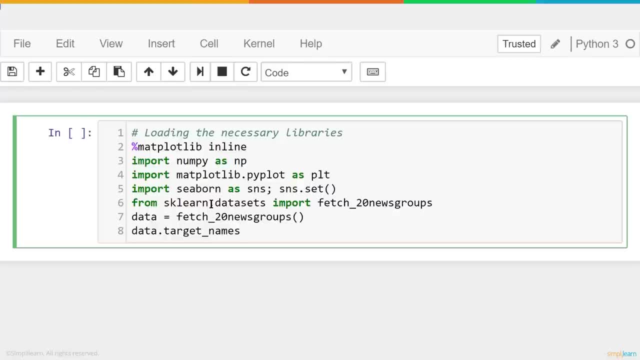 just makes a really nice heatmap. It's really good for heatmaps And if you're not familiar with heatmaps, that just means we give it a color scale. The term comes from the brighter red it is, the hotter. it is in some form of data And you can set it to whatever you want, And we'll see that later. 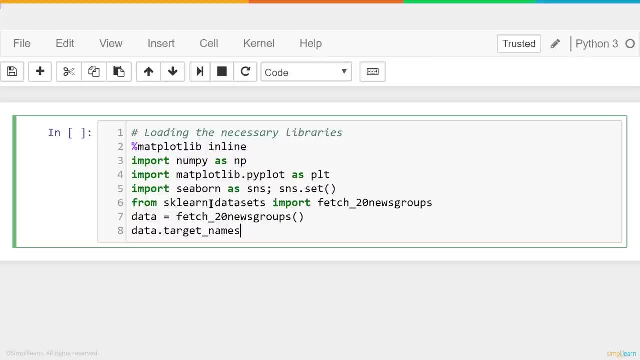 as well. So the next two lines of code here are just importing the graph function so we can graph it, And as a data scientist, you always want to graph your data and have some kind of visual. It's really hard just to shove numbers in front of people and they look at it and it doesn't mean. 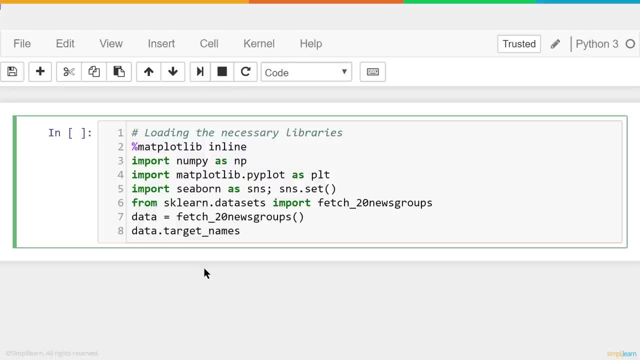 anything. And then from the sklearndatasets we're going to import the fetch20newsgroups- Very common one for analyzing, tokenizing words and setting them up and exploring how the words work and how do you categorize different things when you're dealing with documents. And then we set our 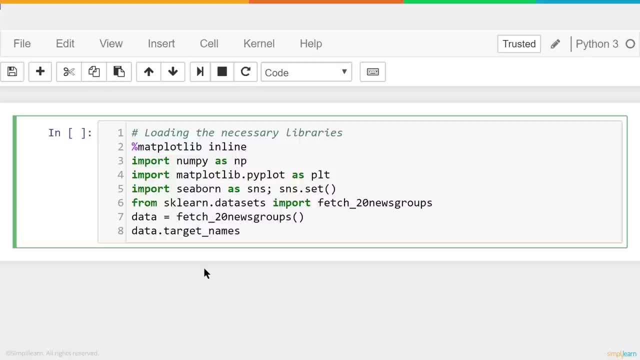 data equal to fetch20newsgroups, And then we set our data equal to fetch20newsgroups, And then we set our data equal to fetch20newsgroups. So our data variable has the data in it and we're going to go. 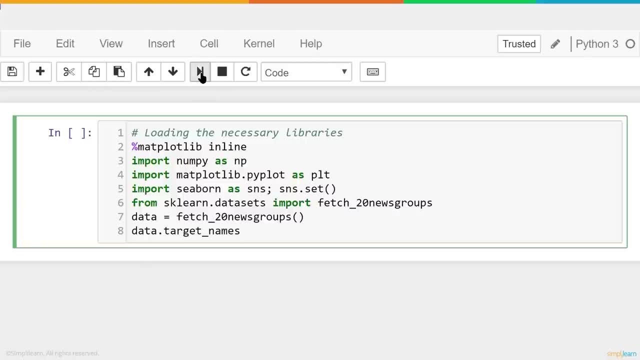 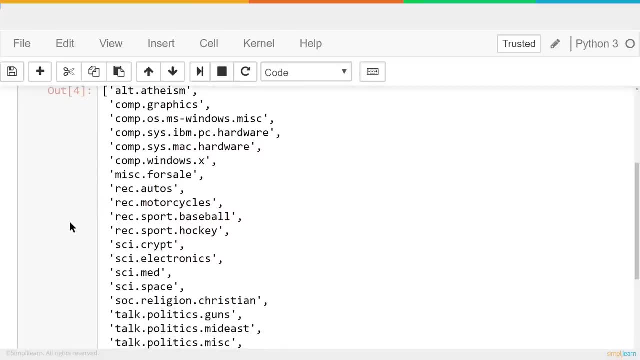 ahead and just print the target name, the datatargetName, And let's see what that looks like. And you see, here we have ALT-Atheism, COMP-Graphics, knowledge&command- resiliency, Comp-OS, ms-windowsmiscellaneous, and it goes down. 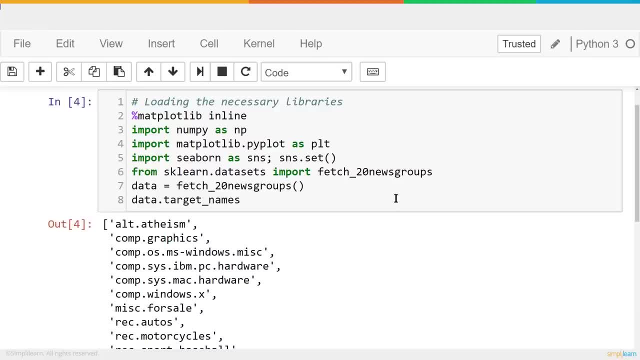 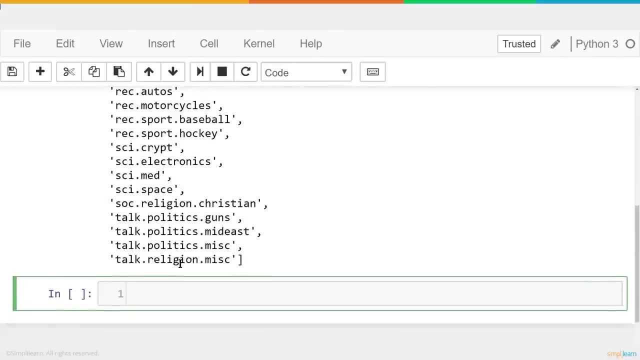 These are the categories we've already assigned to this newsgroup And it's called fetch20 because you'll see, I believe there are 20 different topics or 20 different categories in here as we scroll down. Now we've gone through the 20 different categories and we're going to go ahead. 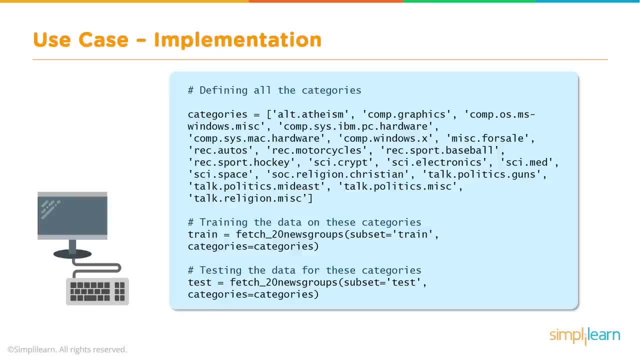 and start defining all the categories and set up our data. So we're actually getting here going to go ahead and get the data all set up and take a look at our data and let's move this over to our Jupyter notebook and let's see what this code does. First, we're going to set our categories. Now, 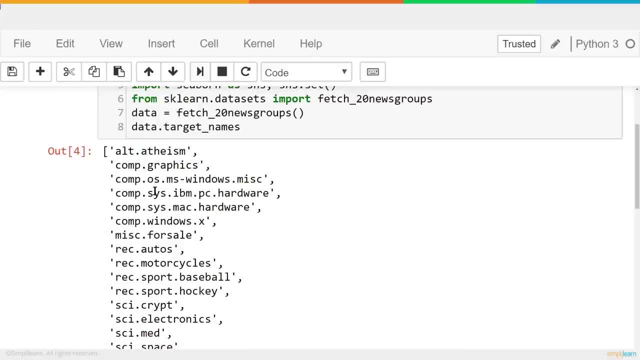 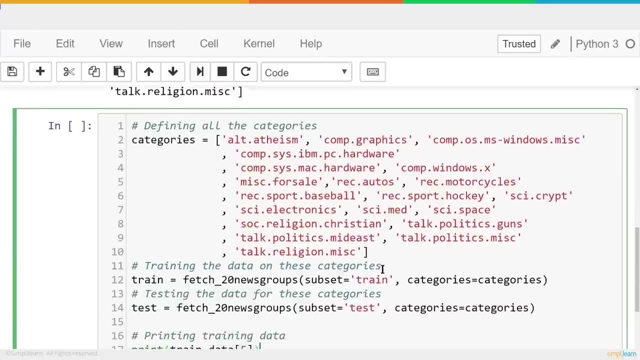 if you noticed up here, I could have just as easily set this equal to datatarget underscore names, because it's the same thing. but we want to kind of spell it out for you so you can see the different categories. It kind of makes it more visual so you can see what your data is looking like in the 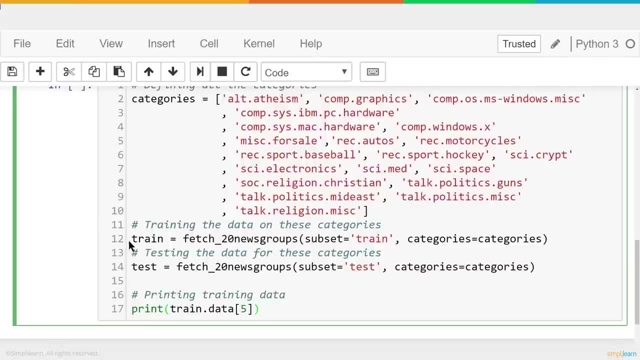 background. Once we've created the categories, we're going to open up a train set. So this training set of data is going to go into fetch 20 news groups and it's a subset in there called train and categories equals categories. So we're pulling out those categories that match and then, if you 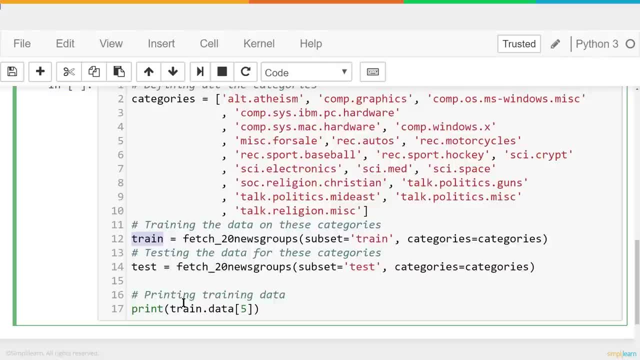 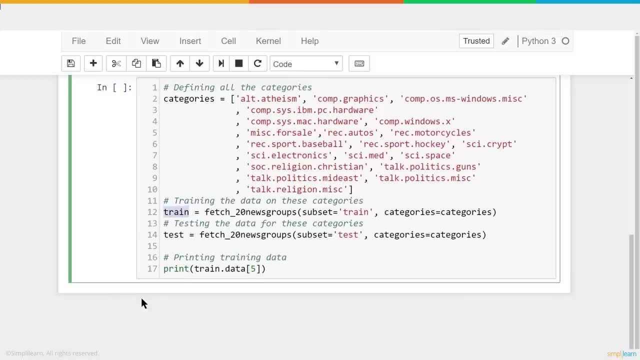 have a train set. you should also have the testing set. We have test equals fetch 20 news groups, subset equals test And categories equals categories. Let's go down one size so it all fits on my screen. There we go, And just so we can really see what's going on, let's see what happens when we print out one part of. 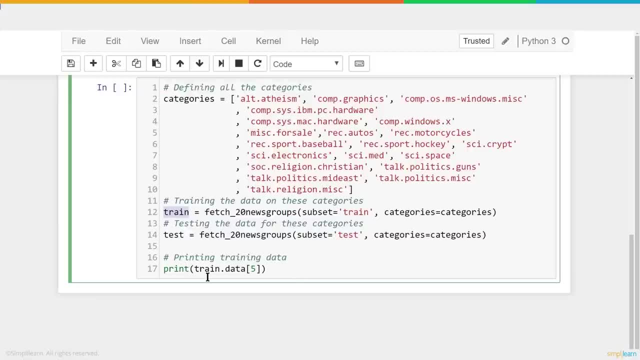 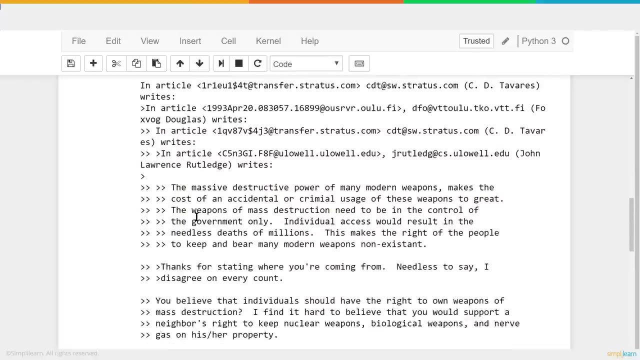 that data. So it creates train and under train it creates train dot data. and we're just going to look at data piece number five And let's go ahead and run that and see what that looks like. And you can see, when I print train dot data number five under train, it prints out one of the articles. This is: 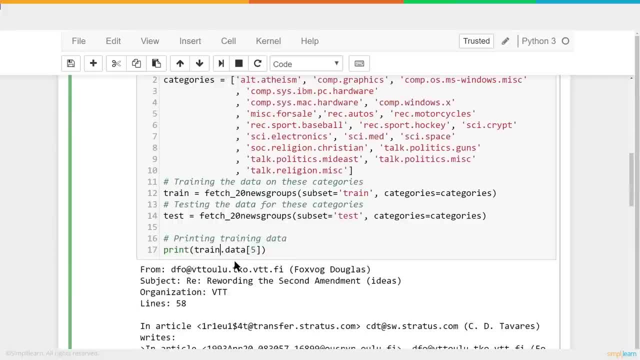 article number five. You can go through and read it on there And we can also go in here and change this to test, which should look identical because it's splitting the data up into different groups. Train and test And we'll see test. number five is a different article, but it's another article in here And maybe you're curious. 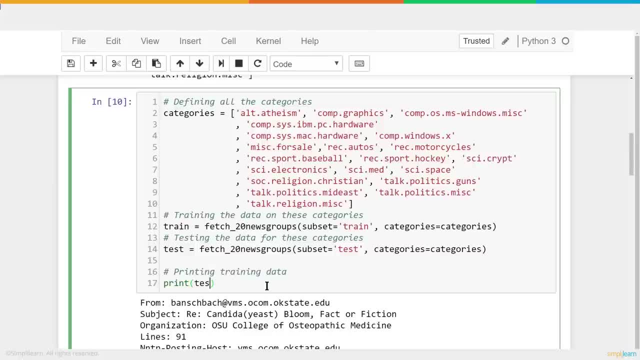 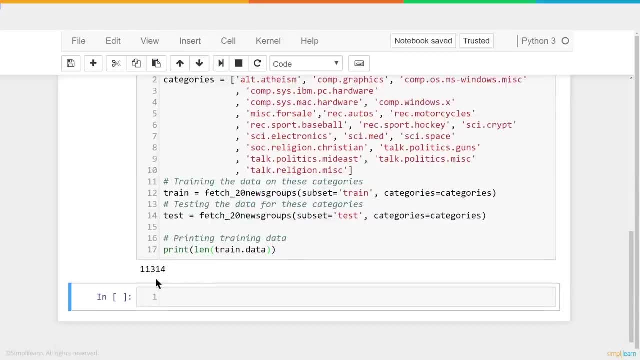 and you want to see just how many articles are in here. We could do length of train dot data And if we run that you'll see that the training data has eleven thousand three hundred and fourteen articles. So we're not going to go through all those articles. That's a lot of articles, But we can look at one of them just to see what kind of 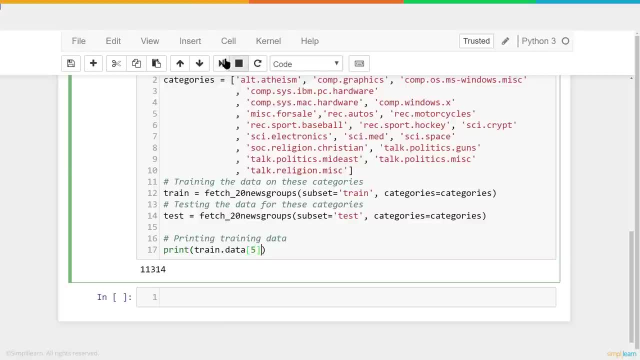 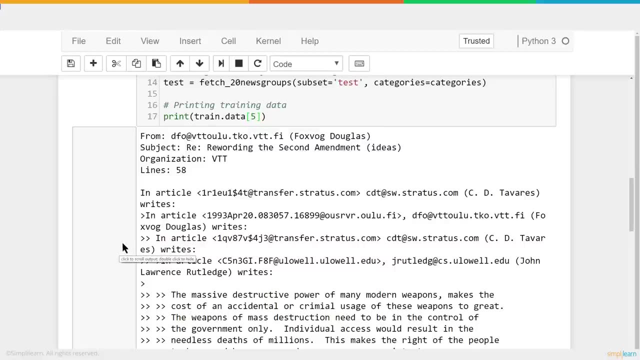 information is coming out of it and what we're looking at. And we'll just look at number five for today. And here we have it, rewording the second amendment: IDs VTT, line fifty eight, lines fifty eight in article Etc, And you scroll all the way down and see all the different parts to there. 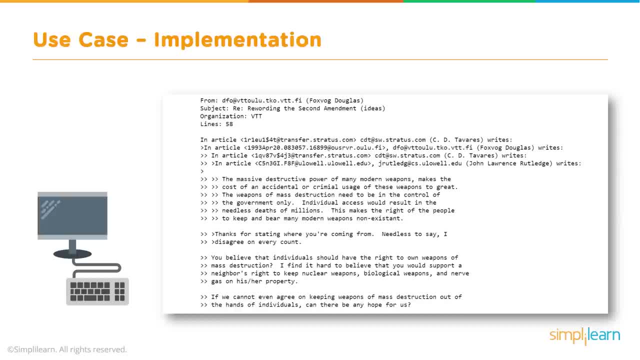 Now we've looked at it and that's pretty complicated when you look at one of these articles to try to figure out how do you weight this. If you look down here, we have different words and maybe the word from Now from, is probably in all the articles, so it's not going to have a lot of meaning as far as trying to figure out whether this article fits one of the categories or not. 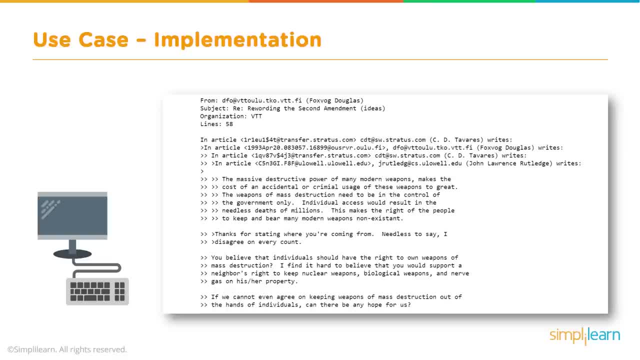 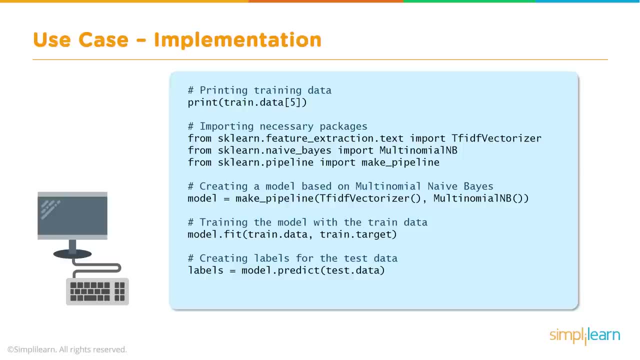 So trying to figure out which category fits in based on these words is where the challenge comes in. Now that we've viewed our data, we're going to dive in and do the actual predictions. This is the actual naive Bayes- And we're going to throw another model at you or another module at you here in just a second. 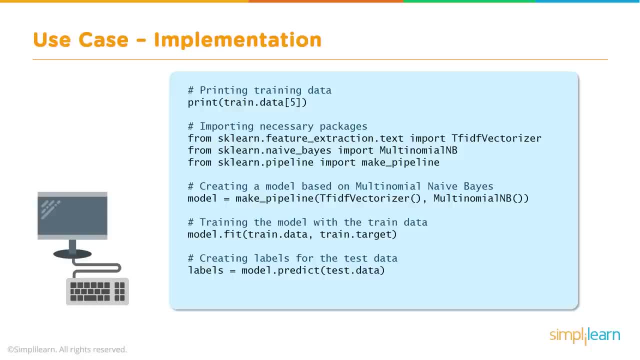 We can't go into too much detail, but it deals specifically working with words and text and what they call tokenizing those words. So let's take this code and let's skip on over to our Jupyter notebook and walk through it And here we are, in our Jupyter notebook. Let's paste that in there. 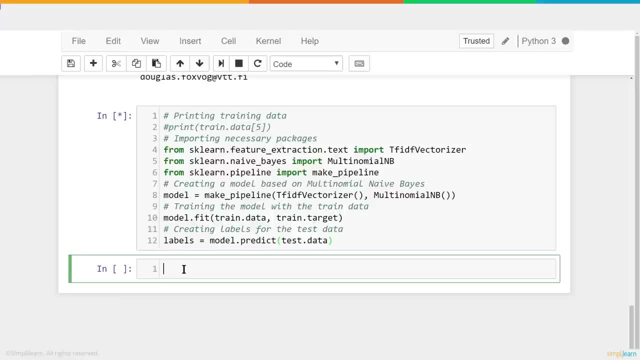 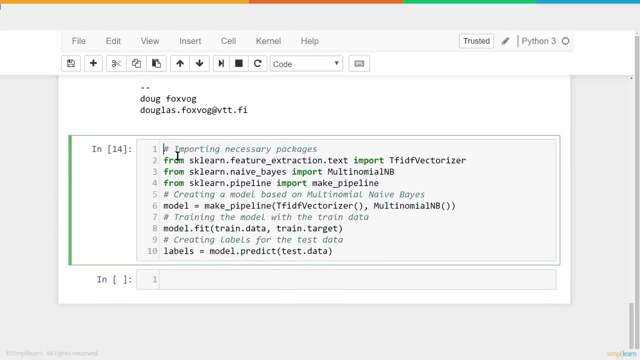 And I can run this code right off the bat. It's not actually going to display anything yet, But it has a lot going on in here. So at the top we have the print module from the earlier one. I didn't know why that was in there. 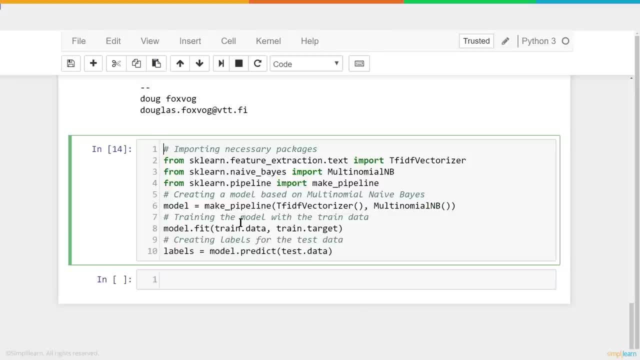 So we're going to start by importing our necessary packages And from the sklearnfeaturesextractiontxt, we're going to import tfidfvn- tfidfvn. I told you that we're going to throw a module at you. We can't go too much into the math behind this or how it works. You can look it up. The notation for the math is usually tfidf. 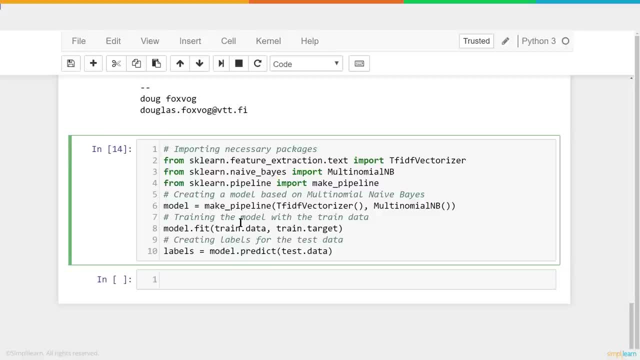 And that's just a way of weighing the words, And it weighs the words based on how many times are used in a document, how many times or how many documents are used in. It's a well used formula. It's been around for a while. It's a little confusing to put this in here. 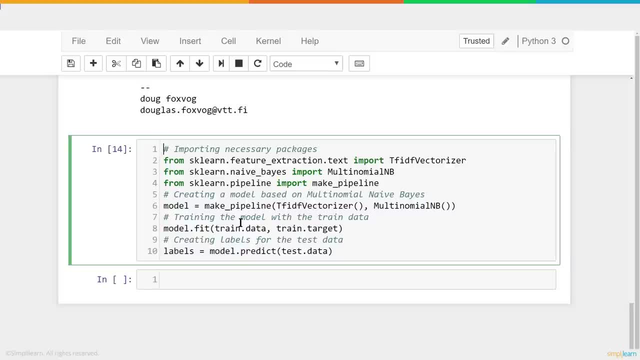 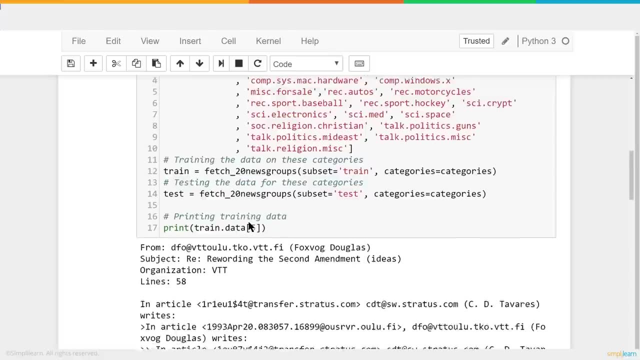 But let's let it know that it just goes in there and weights the different words you need in the document for us. That way we don't have to wait and if you put a wait on it- if you remember I was talking about that up here earlier- if these are all emails, they. 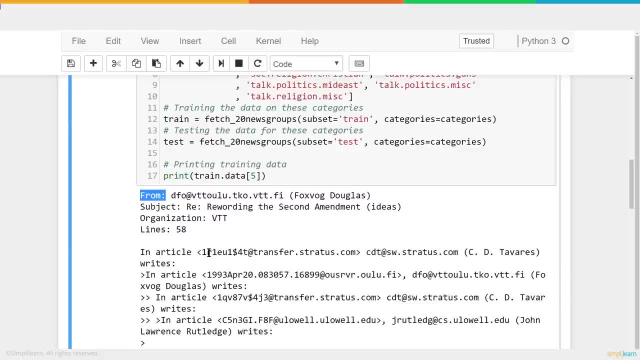 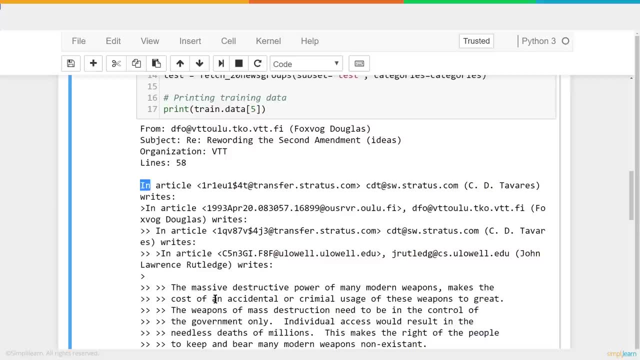 probably all have the word from in them. From probably has a very low weight. It has very little value in telling you what this document's about. Same with words like in, in article, in articles in cost of, on maybe, cost might, or where words like criminal weapons destruction. 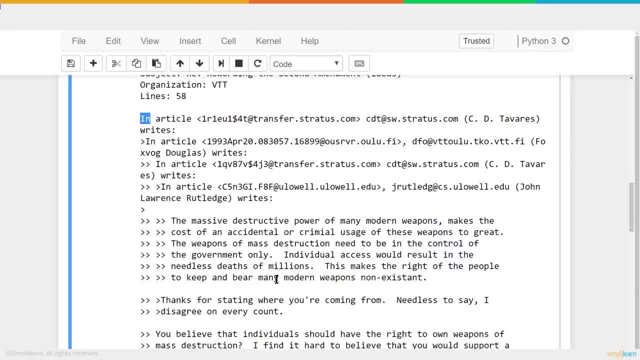 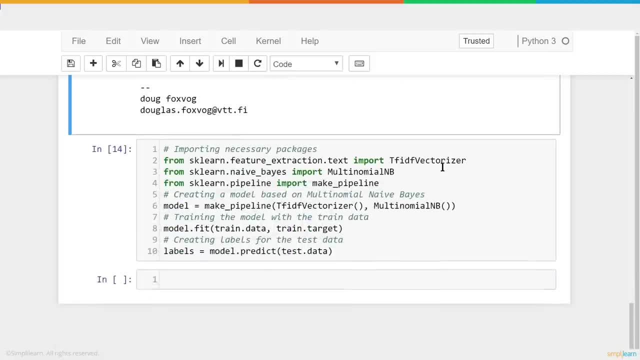 these might have a heavier weight because they describe a little bit more what the article's doing. Well, how do you figure out all those weights in the different articles? That's what this module does. That's what the TF-IDF vectorizer is going to do for us. And then 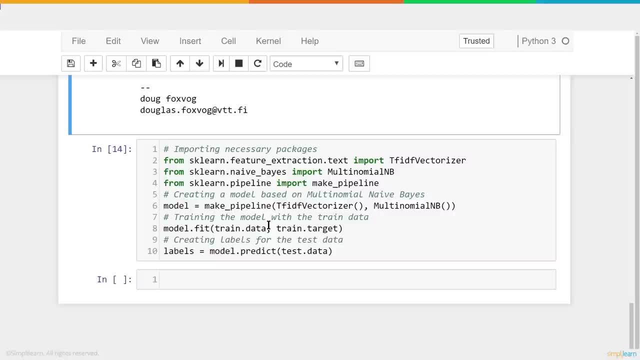 we're going to import our sklearnnaivebase and that's our multinomial NB, Multinomial naive base. pretty easy to understand that where that comes from. And then, finally, we have the sklearn pipeline, import make pipeline. Now, the make pipeline is just a cool piece. 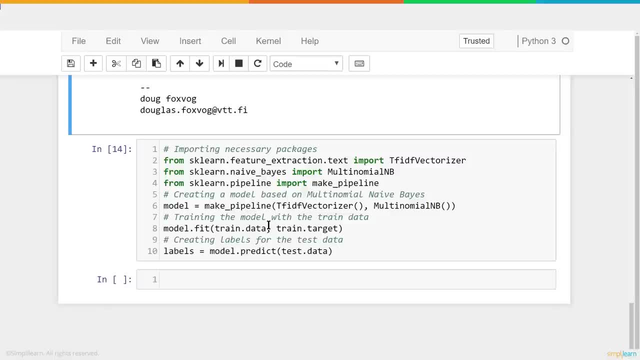 of code because we're going to take the information we get from the TF-IDF vectorizer and we're going to pump that into the multinomial NB. So a pipeline is just a way of organizing how things flow. It's used commonly. you've probably 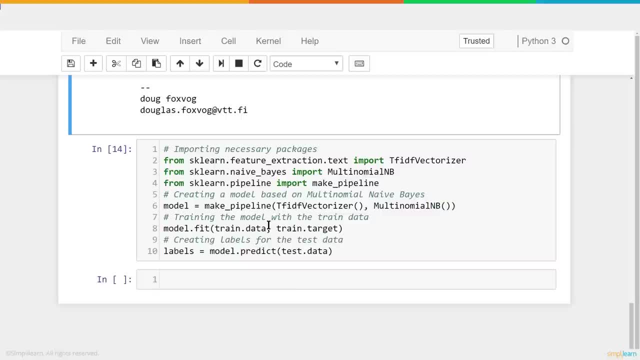 already guessed what it is. If you've done any businesses, they talk about the sales pipeline. If you're on a work crew or a project manager, you have your pipeline of information that's going through or your projects and what has to be done, in what order That's. 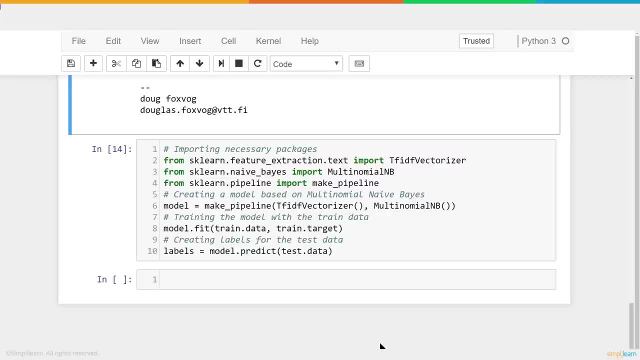 all this pipeline is. We're going to take the TF-IDF vectorizer and then we're going to push that into the multinomial NB. Now we've designated that as the variable model. We have our pipeline model and we're going to take that model and this. 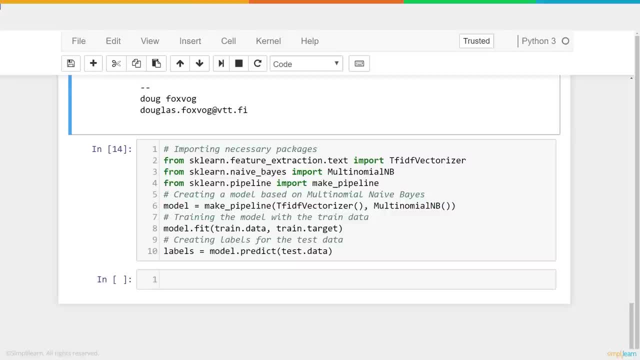 is just so elegant. this is done in just a couple lines of code- Modelfit- and we're gonna fit the data, and first the train data and then the train target. Now the train data has the different articles in it. You can see the one we 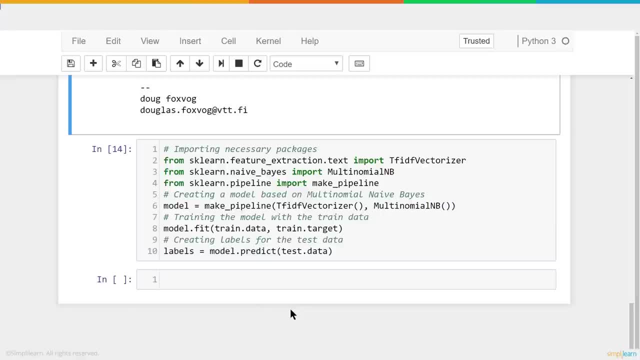 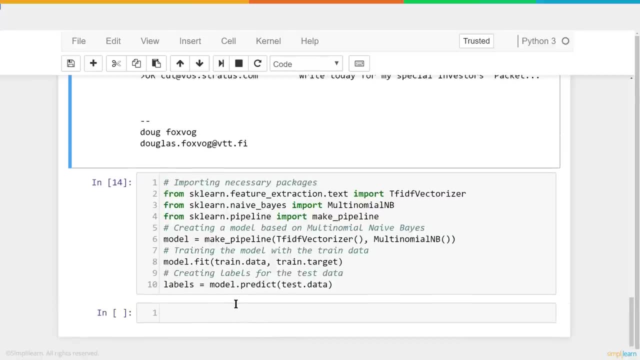 were just looking at and the traintarget is what category they already categorize that that particular article as. And what's happening here is the train data is going into the TF ID vectorizer. So when you have one of these articles, it goes in there, it weights all the words in there. so there's thousands. 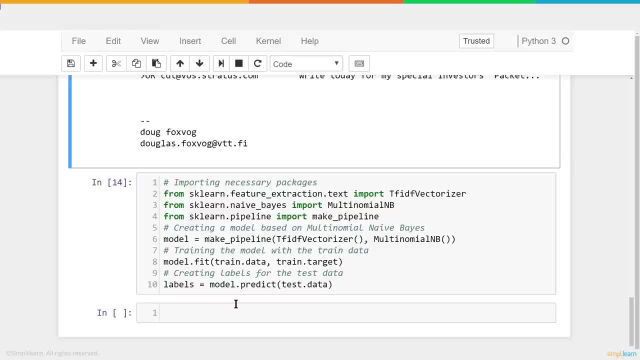 of words with different weights on them. I remember once running a model on this and I literally had 2.4 million tokens go into this. So when you're dealing like large document bases, you can have a huge number of different words. It then takes those words, gives them a weight and then 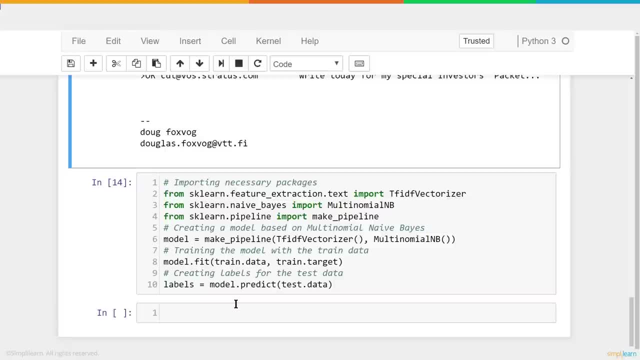 based on that weight, based on the words and the weights, and then puts that into the multinomial NB, And once we go into our naive base we want to put the train target in there. so the train data that's been mapped to the TF ID vectorizer is now going through the multinomial NB and then we're telling it: 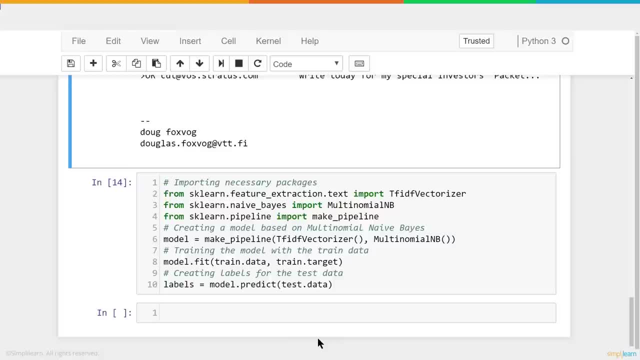 well, these are the answers. These are the answers to the different documents. So this document that has all these words, with these different weights from the first part is going to be, whatever category it comes out of- Maybe it's the talk show or the article on religion- miscellaneous, Once we fit that. 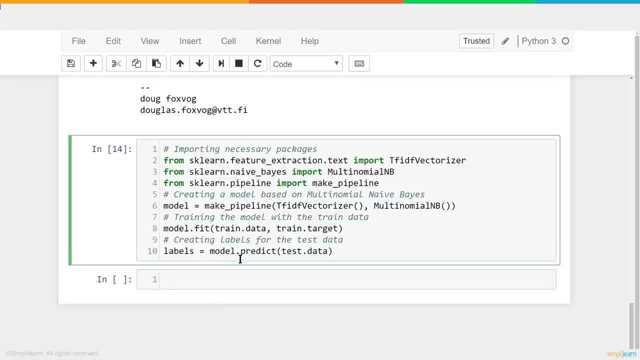 model. we can then take labels and we're going to set that equal to model dot predict. Most of the sklearn use the term dot predict to let us know that we've now trained the model and now we want to get some answers. We're going to 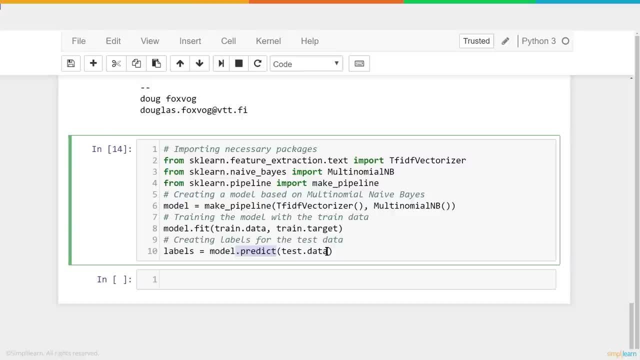 put our test data in there, because our test data is the stuff we held off to the side, We didn't train it on there and we don't know what's going to come up out of it, and we just want to find out how good our labels are. 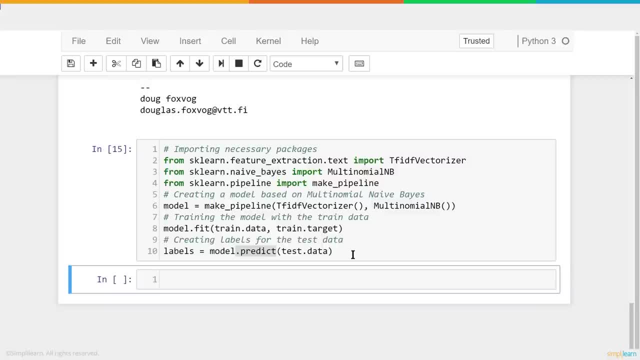 Do they match what they should be? Now, I've already run this through. There's no actual output to it to show. This is just setting it all up. This is just training our model, creating the labels, so we can see how good it is. 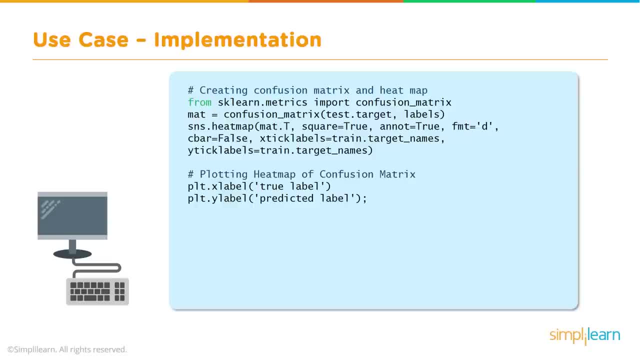 and then we move on to the next step: to find out what happened. To do this, we're going to go ahead and create a confusion matrix and a heat map. So the confusion matrix, which is confusing just by its very name, is basically going to ask: how confused is our answer? 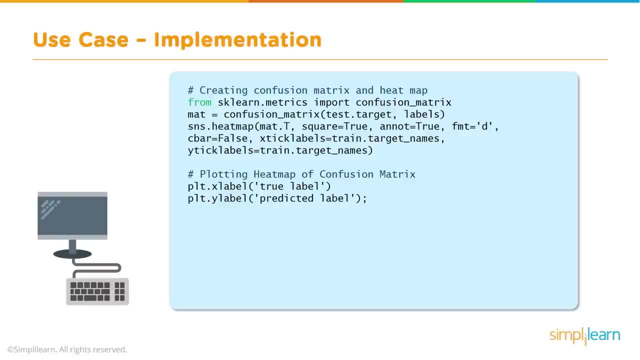 Did it get it correct or did it miss some things in there or have some missed labels, And then we're going to put that on a heat map, so we'll have some nice colors to look at. to see how that plots out, Let's go ahead and take this code and take a walk through it and see what that looks like. 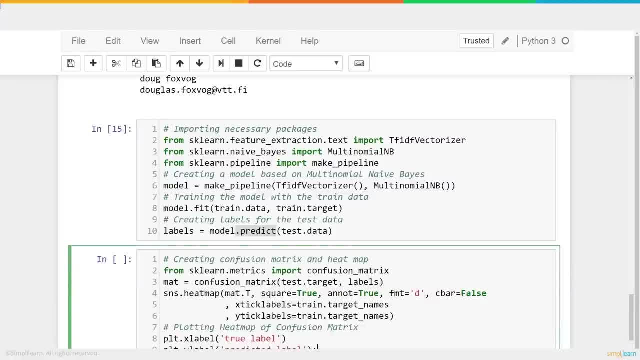 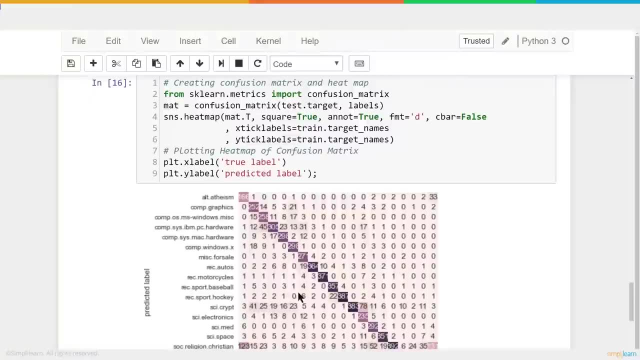 So back to our Jupyter notebook. I'm going to put the code in there and let's go ahead and run that code. Take it just a moment And remember we had the inline. That way my graph shows up on the inline. 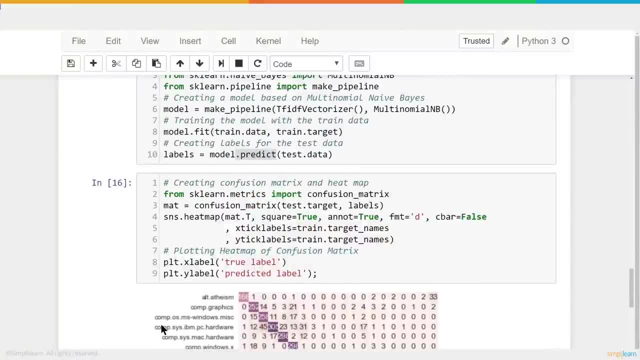 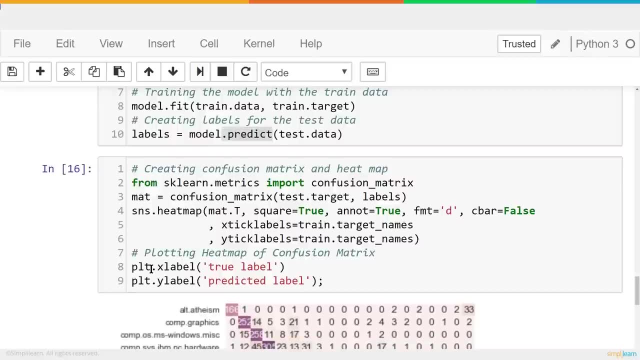 And let's walk through the code and then we'll look at this and see what that means. So let me make it a little bit bigger. There we go, No reason not to use the whole screen Too big. So we have here from sklearnmetrics import confusion matrix. 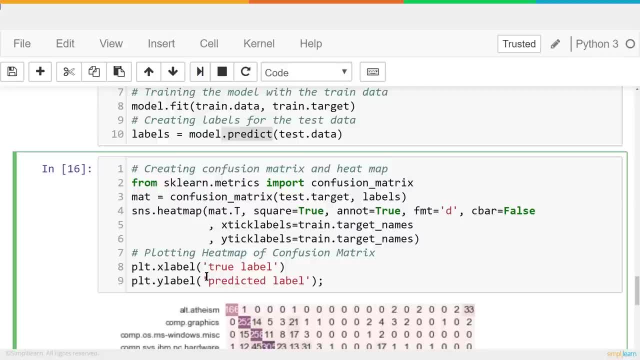 And that's just going to generate a set of data that says the prediction was such. the actual truth was either agreed with it or it was something different. And it's going to add up those numbers so we can take a look and just see how well it worked. 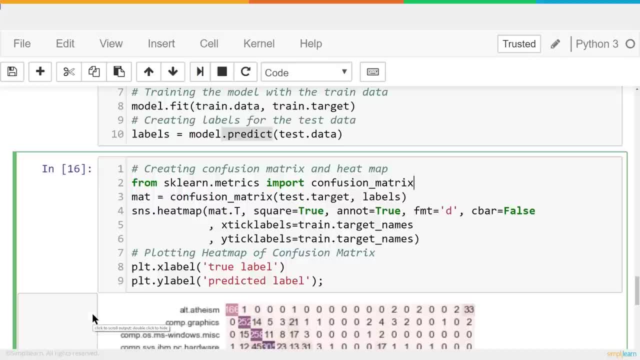 And we're going to set a variable Mat equal to confusion matrix. We have our test target, our test data. that was not part of the training- Very important in data science. we always keep our test data separate, Otherwise it's not a valid model if we can't properly test it with new data. 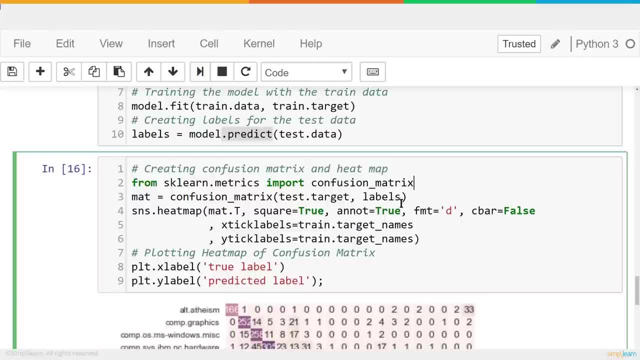 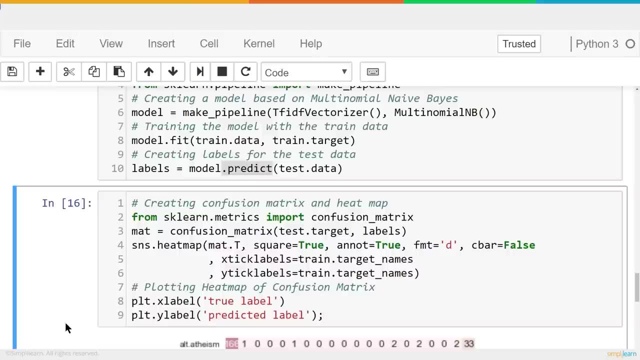 And this is the labels we created from that test data. These are the ones that we predict it's going to be. So we go in and we create our SN heat map. The SNS is our seaborne, which sits on top of the pi plot. 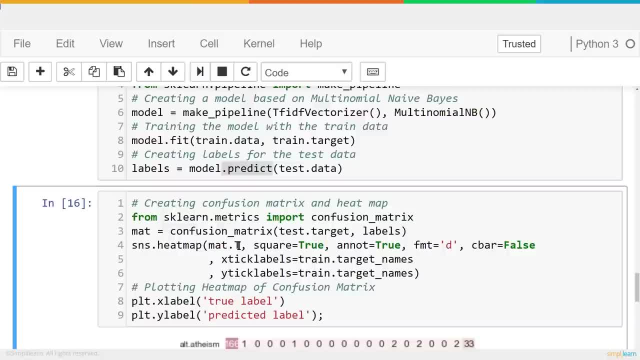 So we create a SNSheat, We take our confusion matrix and it's going to be matt- And do we have other variables that go into the SNSheat map? We're not going to go into detail what all the variables mean. 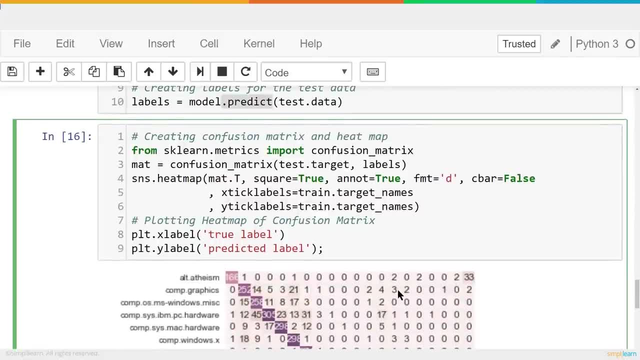 The annotation equals true. that's what tells it to put the numbers here. So you have the 166, the 1, the 0001.. Format D and the C bar equals false. have to do with the format. If you take those out, you'll see that some things disappear. 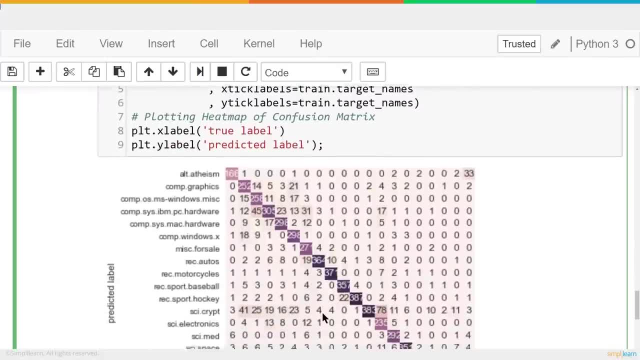 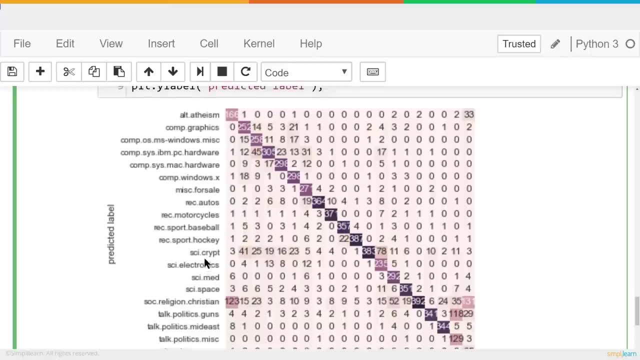 And then the X tick labels and the Y tick labels. Those are our target names And you can see right here: that's the alt atheism, comp, graphics, comp, osms, windowsmiscellaneous. And then finally, we have our pltxlabel. 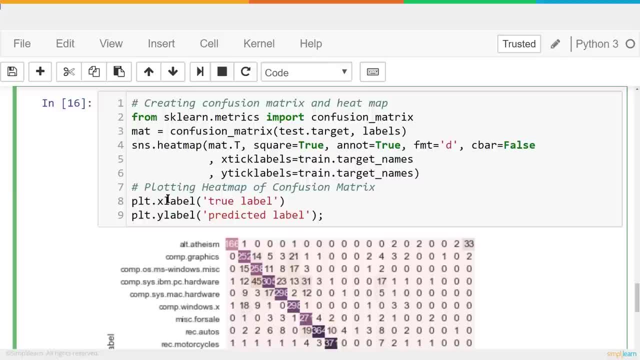 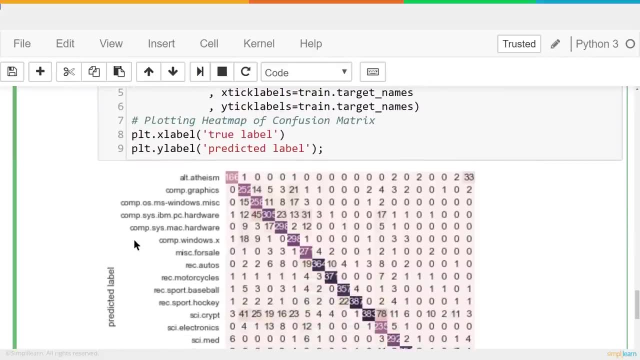 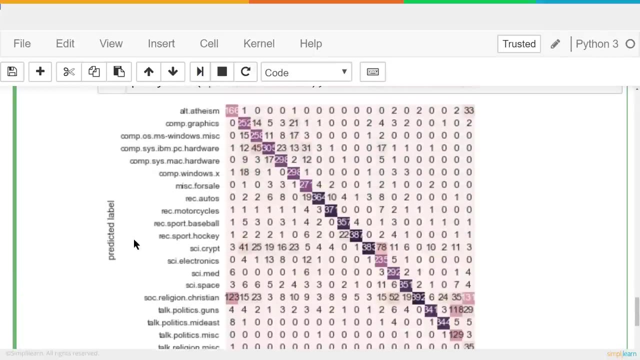 Remember the SNS or the seaborne sits on top of our matplot library, our plt, And so we want to just tell it: xlabel equals a true is true, The labels are true. And then the Y label is prediction label. So when we say a true, this is what it actually is and the prediction is what we predict. 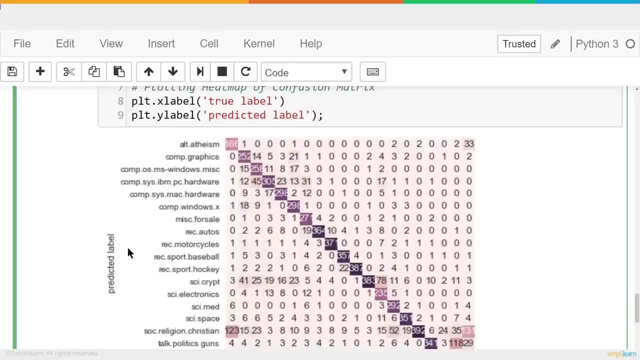 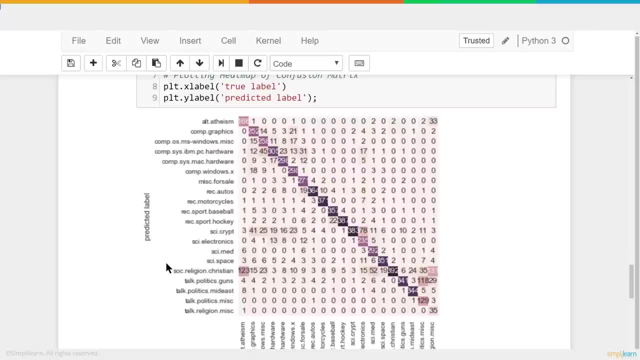 And let's look at this graph, because that's probably a little confusing the way we rattled through it, And what I'm going to do is I'm going to go ahead and flip back to the slides because they have a black background they put in there. that helps it shine a little bit better. so 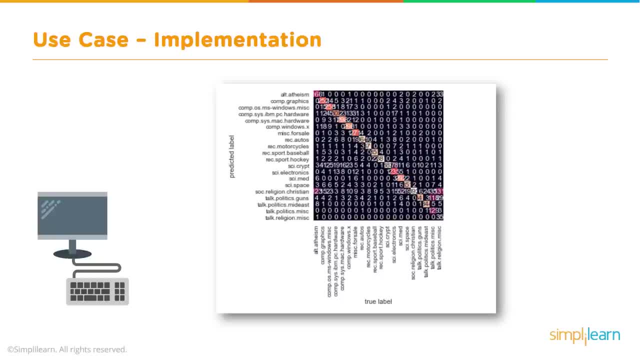 you can see the graph a little bit easier. So in reading this graph, what we want to look at is how the color scheme has come out, And you'll see a line right down the middle diagonally from upper left to bottom right. 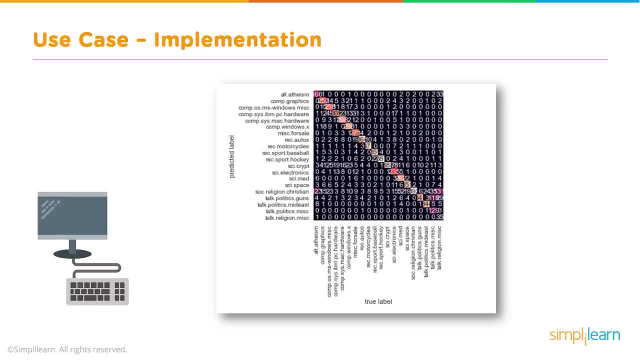 What that is is, if you look at the labels, we have our predicted label on the left and our true label on the right. Those are the numbers where the prediction and the true come together, And this is what we want to see is we want to see those lit up. 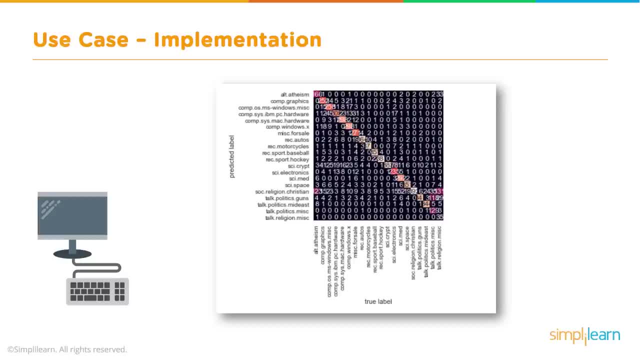 That's what that heat map does is. you can see that it did a good job of finding those data And you'll notice that there's a couple of red spots on there where it missed. You know it's a little confused when we talk about talk, religion, miscellaneous versus talk. 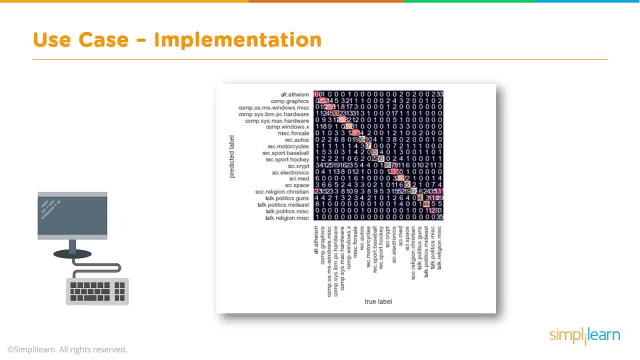 politics, miscellaneous social religion, Christian versus alt atheism. It mislabeled some of those And those are very similar topics. So you can see that there's a lot of mislabeled data And you'll notice that there's a lot of mislabeled data. 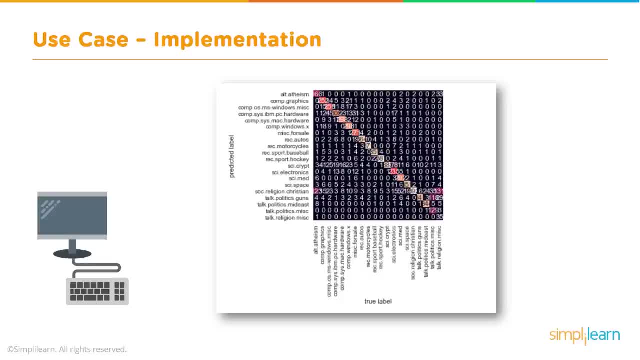 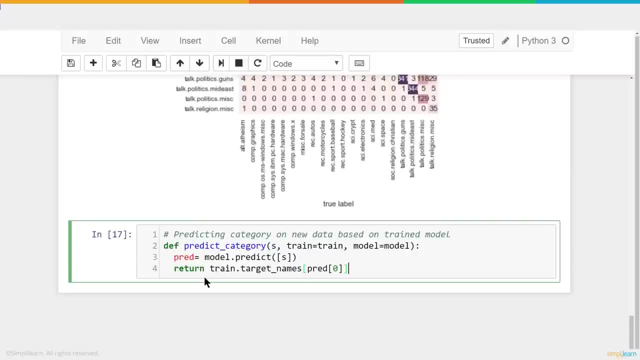 You could understand why it might mislabel them, But overall it did a pretty good job. If we're going to create these models, we want to go ahead and be able to use them, So let's see what that looks like. To do this, let's go ahead and create a definition, a function to run. 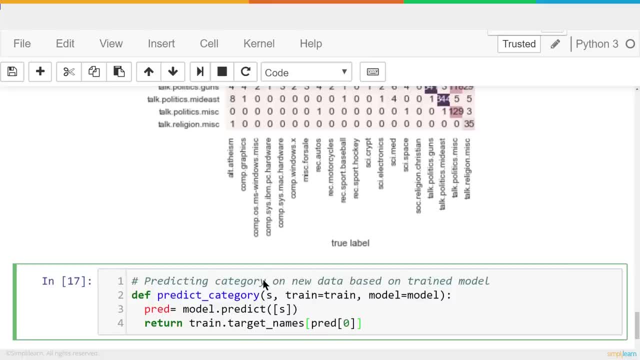 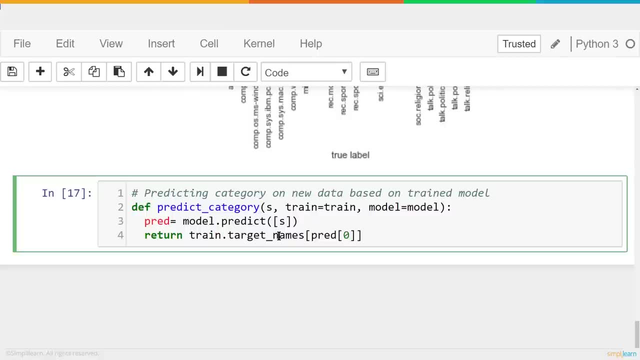 And we're going to call this function. Let me just expand that just a notch here. There we go. I like mine in big letters. Predict categories. We want to predict the category. We're going to send it as a string. 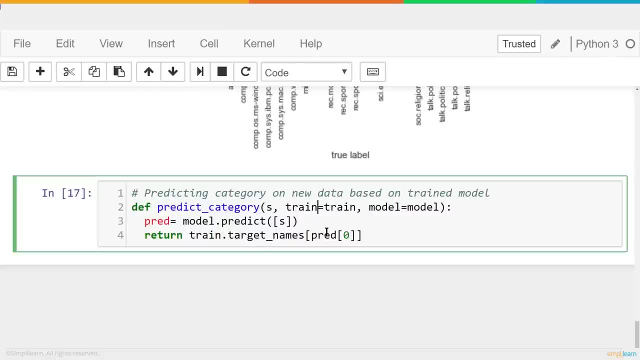 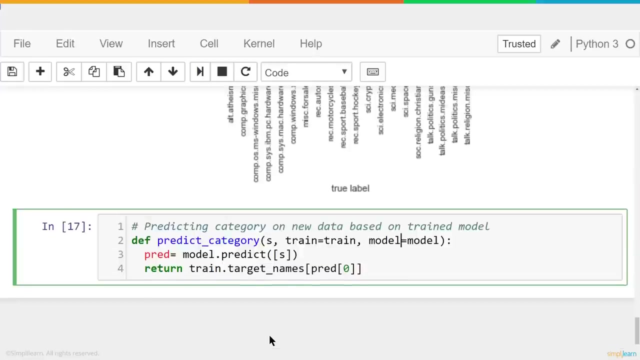 And then we're sending it: train equals train. We have our training model And then we had our pipeline pipeline: Model equals model. This way we don't have to resend these variables each time. The definition knows that, because I said train equals train and I put the equal for model And then we're going to set the prediction equal to the model dot, predict s. So it's going to send whatever string we send to it. It's going to push that string through the pipeline, the model pipeline. It's going to go through and tokenize it and put it through the tf idf, convert that into numbers and weights for all the different documents and words. 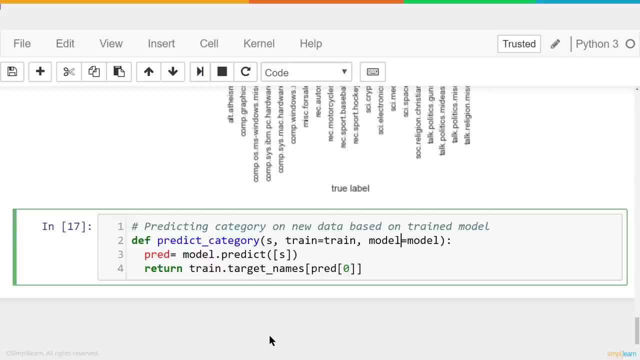 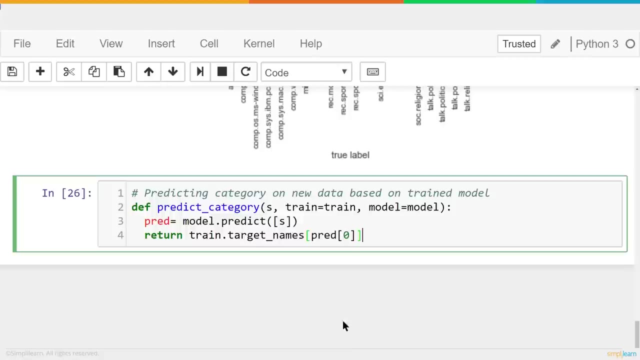 And then it'll put that through our naive bays And from it we'll go ahead and get our prediction. We're going to predict what value it is And so we're going to return train dot target names, predict of zero. And remember that the train dot target names- that's just categories. I could have just as easily put categories in there- dot, predict of zero. So we're taking the prediction, which is a number, and we're converting it to an actual category. We're converting it from. I don't know what the actual numbers are, but let's say zero. 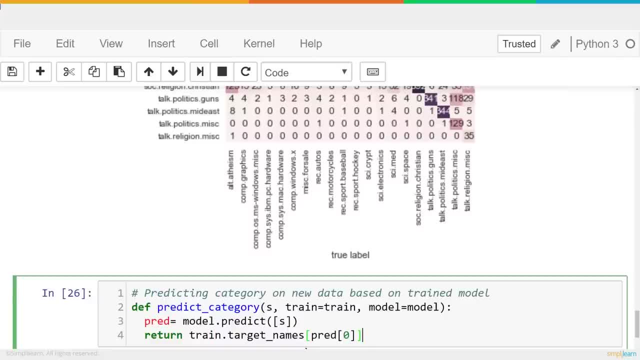 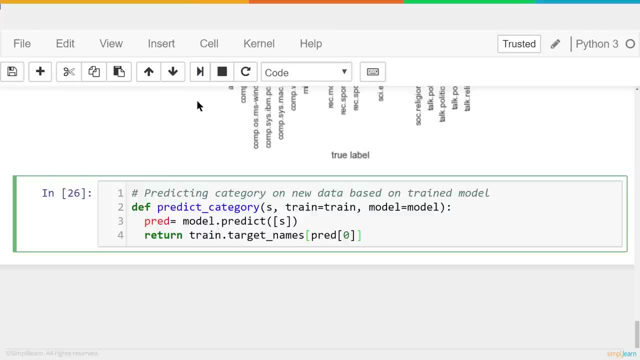 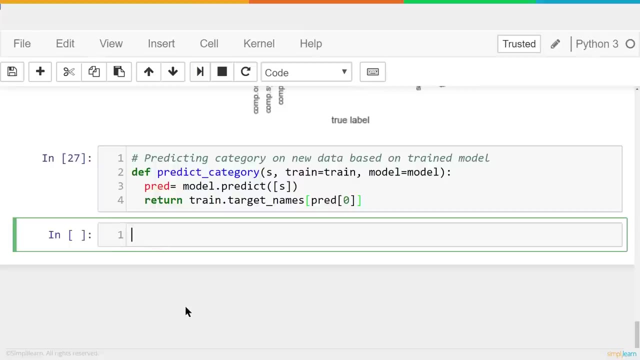 Zero equals alt atheism, So we're going to convert that zero to the word or one. Maybe it equals comp graphics, So we're going to convert number one into comp graphics. That's all that is. And then we got to go ahead and and then we need to go ahead and run this, So I load that up And then, once I run that, we can start doing some predictions. I can go ahead and type in predict category And let's just do predict category Jesus Christ, And it comes back and says it's social religion: Christian. That's pretty good. 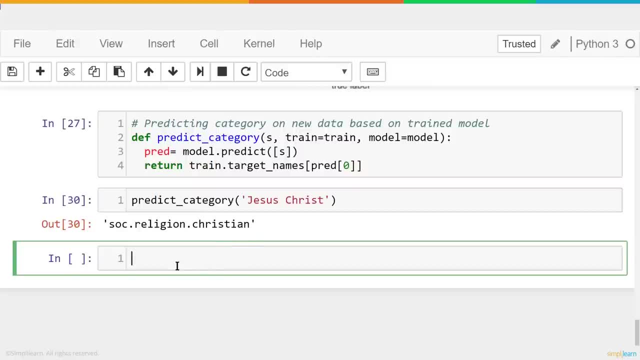 Pretty good. Now note: I didn't put print on this. One of the nice things about the Jupyter notebook editor and a lot of inline editors is if you just put the name of the variable out as returning the variable train dot target underscore names, it'll automatically print that for you In your own ID. you might have to put in print. Let's see where else we can take this. And maybe you're a space science buff. So how about sending load to international space station? 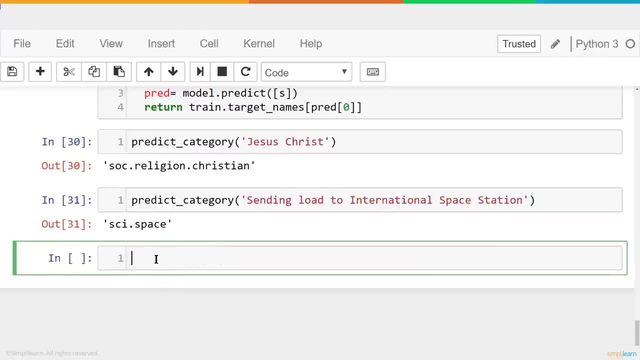 And if we run that we get science, space. Or maybe you're a automobile buff And let's do. they were going to tell me Audi is better than BMW. But I'm going to do, BMW is better than an Audi. So maybe you're a car buff And we run that And you'll see. it says recreational. I'm assuming that's what REC stands for Autos. So I did a pretty good job labeling that one. How about if we have something like a caption running through there? 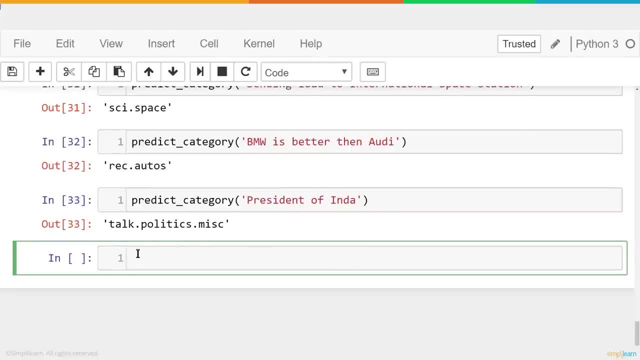 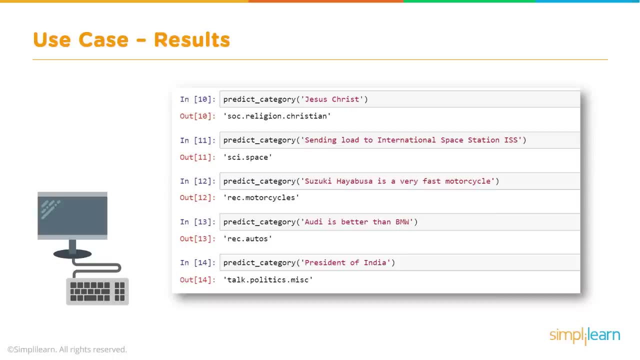 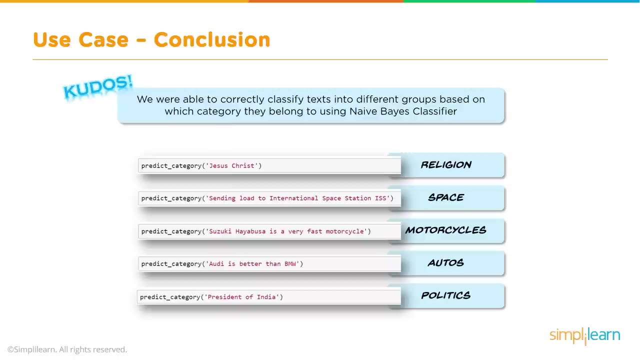 And if we run that, it comes up and says: talk politics miscellaneous. So when we take our definition or our function and we run all these things through kudos- we made it- We were able to correctly classify texts into different groups, based on which category they belong to, using the naive base classifier. Now we did throw in the pipeline the TF idea vectorizer, We threw in the graphs. Those are all things that you don't necessarily have to know.